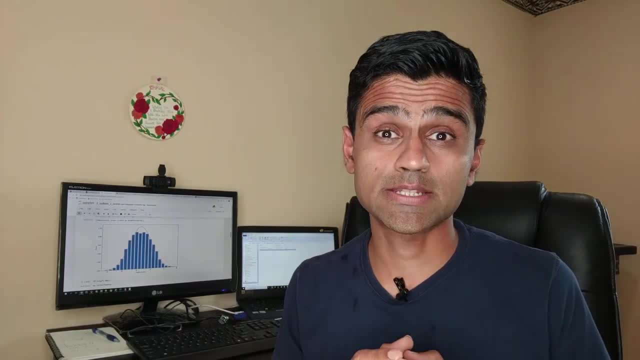 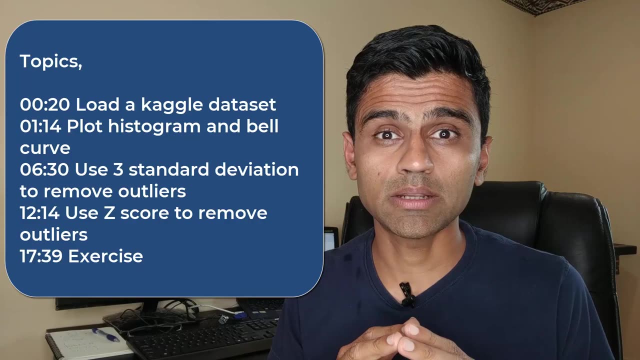 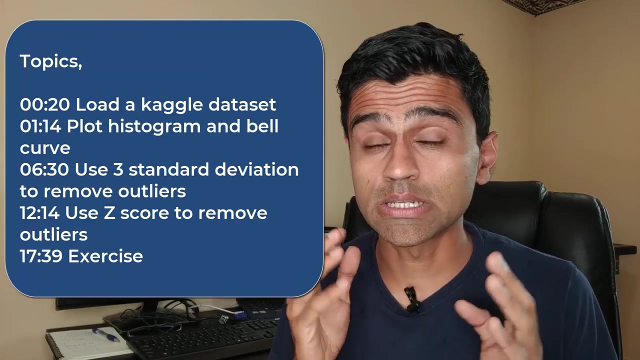 In this video we are going to look at how you can use z-score and standard deviation to remove outliers from your data set. We will be using a real data set from kegelcom and remove outliers using z-score and three standard deviation. In the end, we'll have an interesting exercise for you to 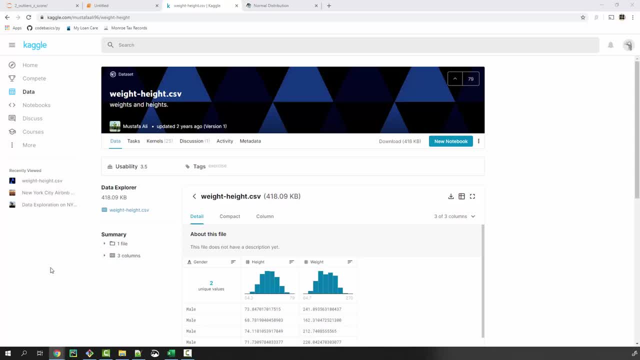 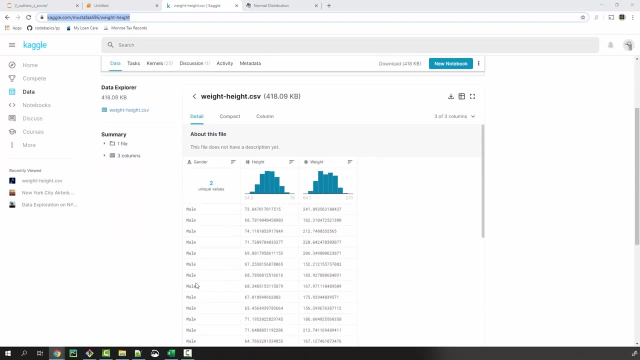 work upon, We will be using weight and height data set from kegel. Thanks, Mustafa Ali, for providing this data set. This data set has height and weight, two columns. It's basically the weight and height of different people And, just to make things simple, I have removed weight from that. 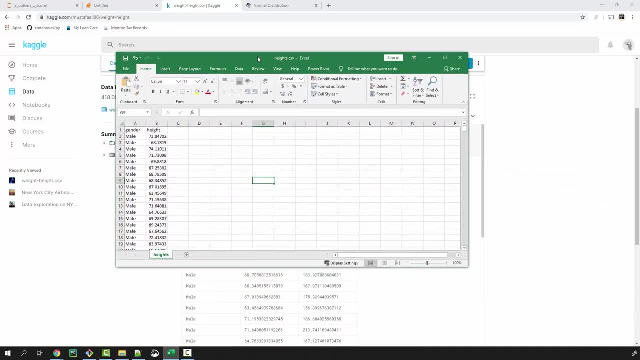 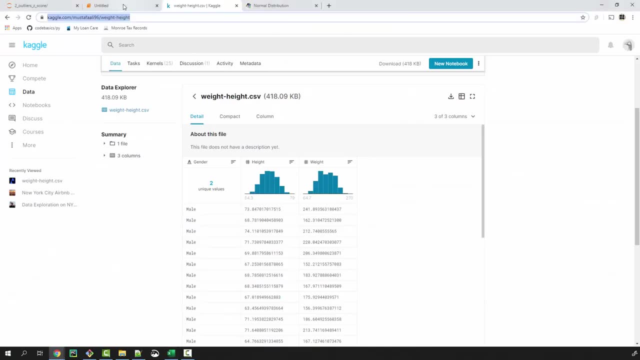 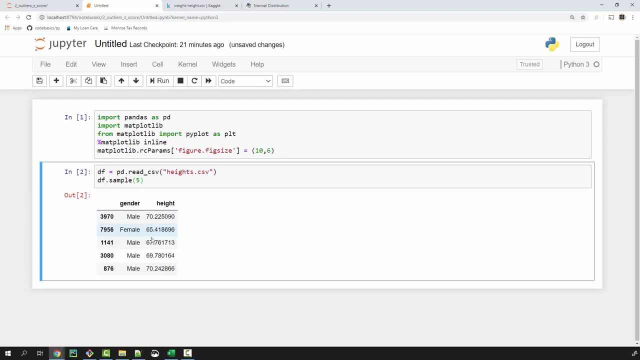 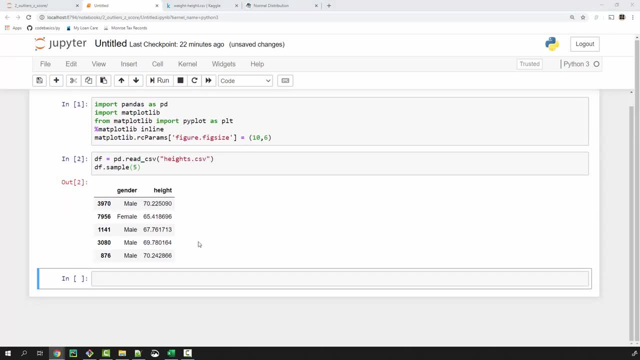 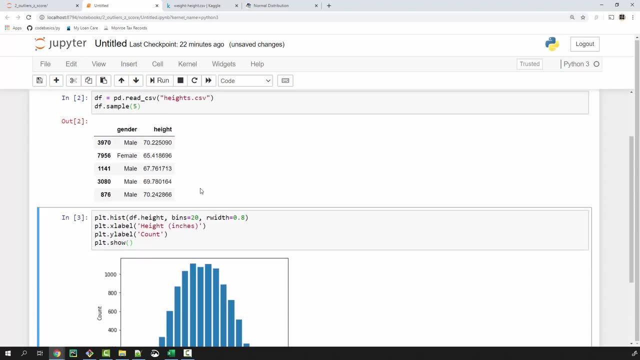 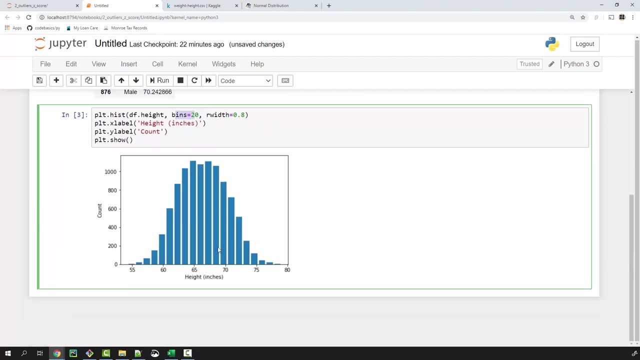 distribution. So the histogram will look something like this. So here you know, I have this height column that I'm using to plot the histogram, and beans is like how many bars that you want to see on the chart. Okay, if you increase the bean size, you'll see. 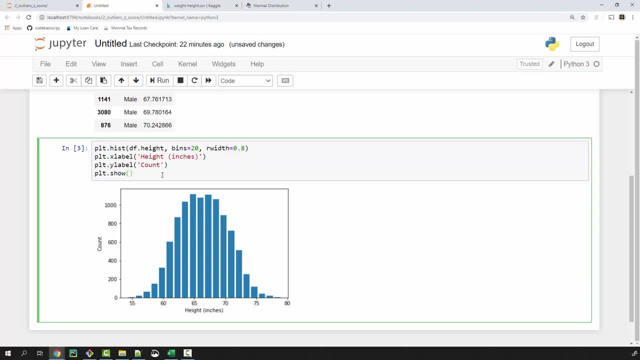 more chart, more beans here. So this histogram shows normal distribution. Now, if you don't know about histograms, this is very simple. Actually, what this is saying is: for 65 inch height, I have more than 1000 samples. For 60 inch height, I have around 370, 300,. 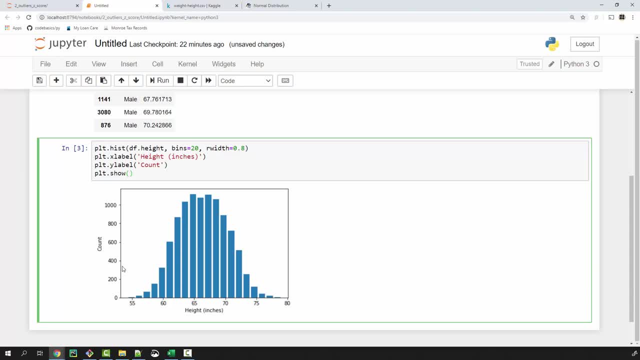 980 samples. So the y axis shows the number of samples that you have in data set for that x value, which is your height. okay, So if you don't know about histogram again, Google it title and get yourself familiar. Once you have the histogram you can figure out if your 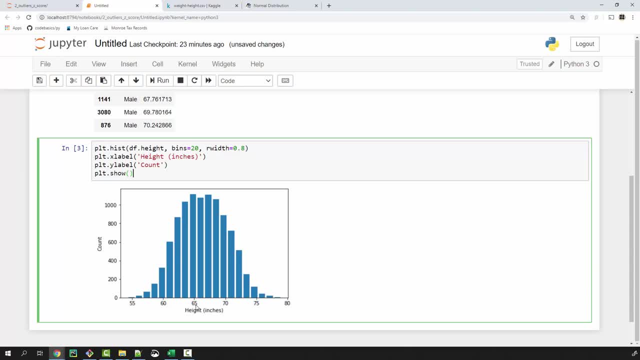 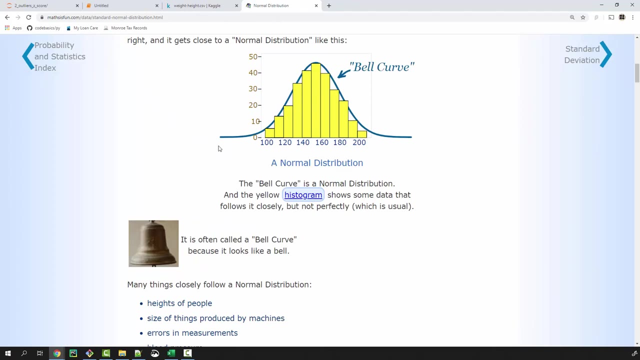 familiar. Once you have the histogram, you can figure out if your distribution is a normal distribution or not. Now, what is a normal distribution? So if you go to this website, mathisfuncom- This is a great website, by the way- This website explains how a normal distribution looks, like It often. 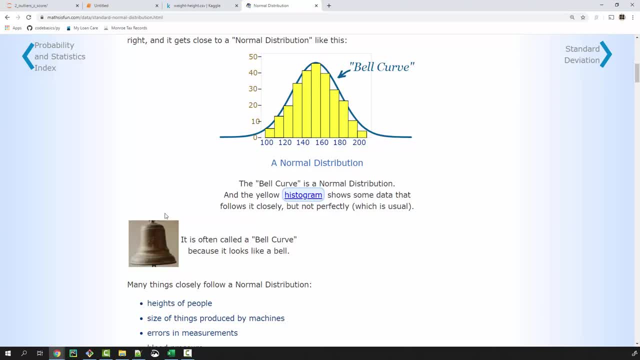 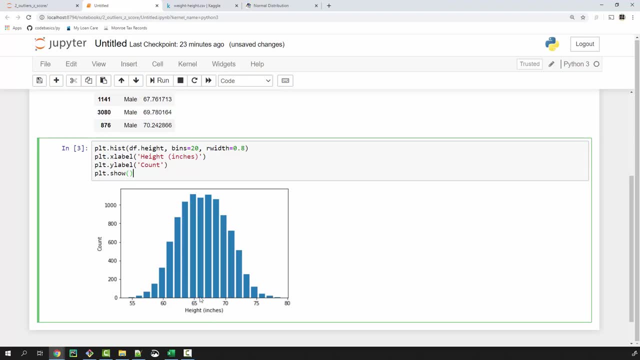 has this shape of a bell curve because it looks like a bell and what it means is majority of the values are centered around mean or an average, and then, as you go away from mean, the number of values goes down In nature. we see many data sets which follow normal distribution, For example, 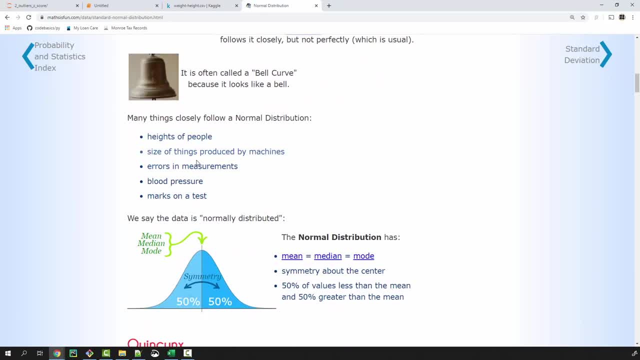 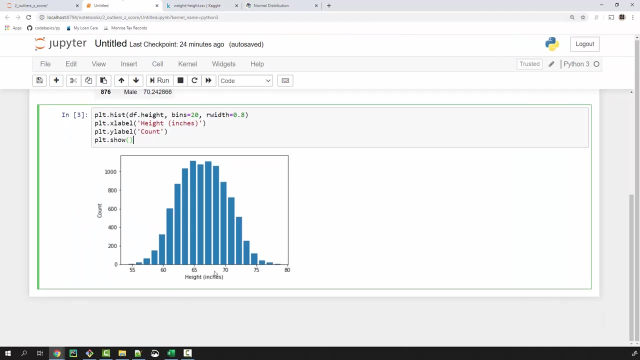 here they are saying heights of the people, size of the things produced by machines. you know, blood pressure, marks on taste. These are all examples of a normal distribution where, if you are taking example of heights of the people, which is this data set, you will notice that majority of the 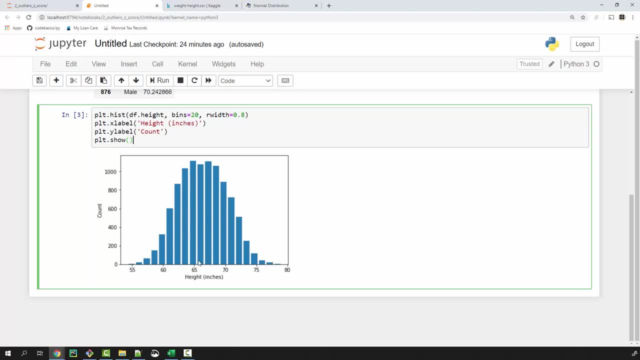 people have heights between you know in this area, 65 to 68 inch, and then people having around 80 inch height, which is more than which is around 7 feet, is very less. so you can see, number of samples are less. similarly, number of people having very less height, which is like 4 feet, 4 feet 5 inch. 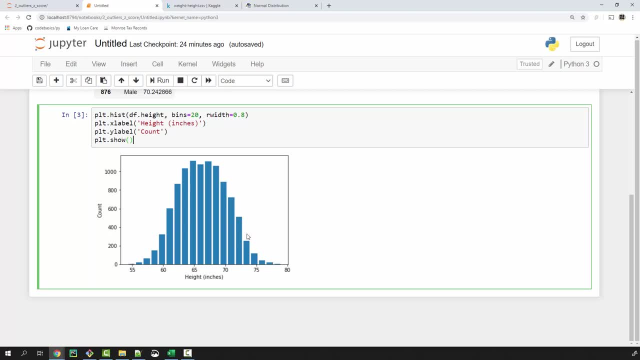 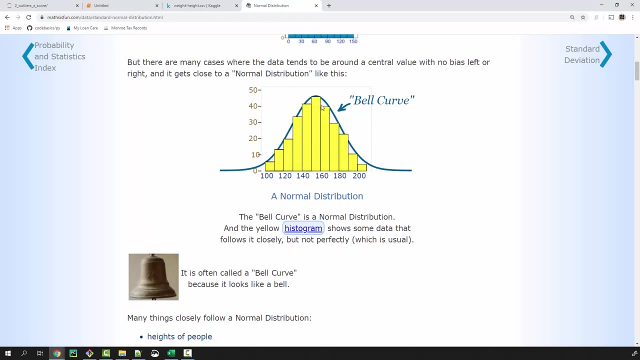 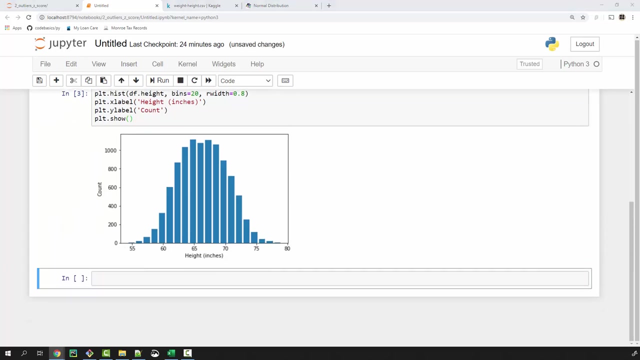 is also less so. this data set is clearly following a normal distribution. now what we're going to do is we will plot a bell curve that you saw here. so this is this yellow chart is a histogram and this curve is a bell curve, and we'll just plot that bell curve for our visualization purpose and you. 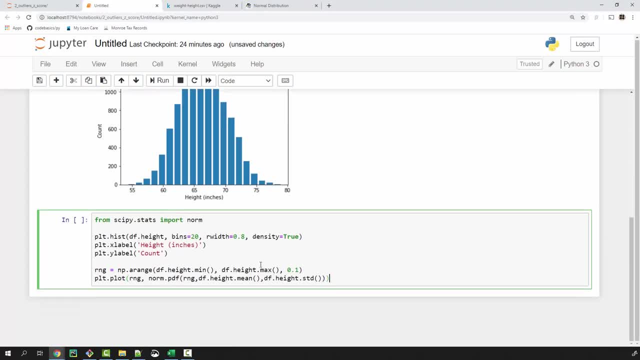 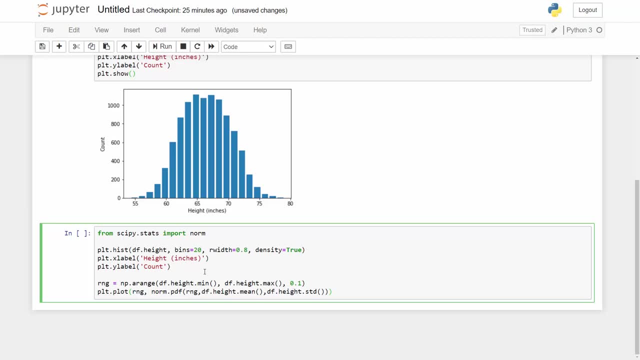 will need to use a scipy module. so if you have installed scipy module already, it, i think, comes with anaconda installation, so you should be good. these three lines are same as this. okay, so you are plotting a histogram here and then in these two lines you are plotting the actual bell curve. 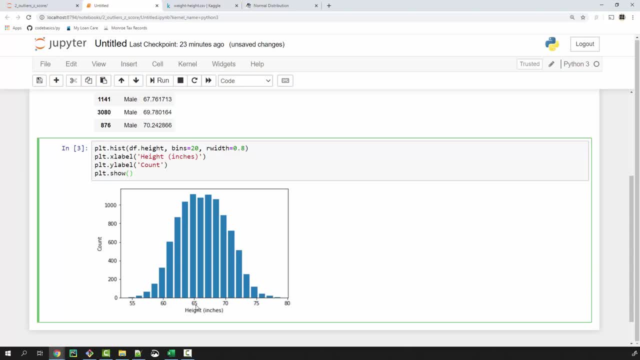 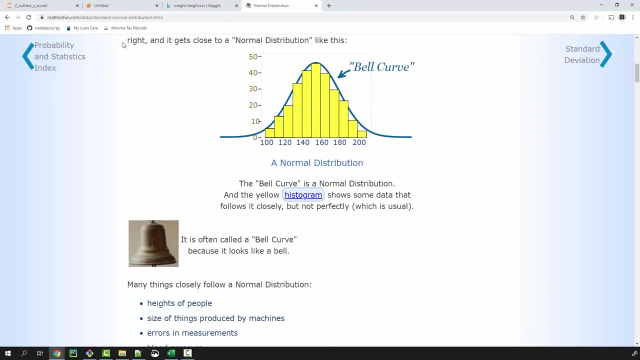 distribution is a normal distribution or not? Now, what is a normal distribution? So, if you go to this website, mathisfuncom, destination, H2O, SEED x data set that You can choose is a great website. by the way, this website explains how a normal distribution looks like. 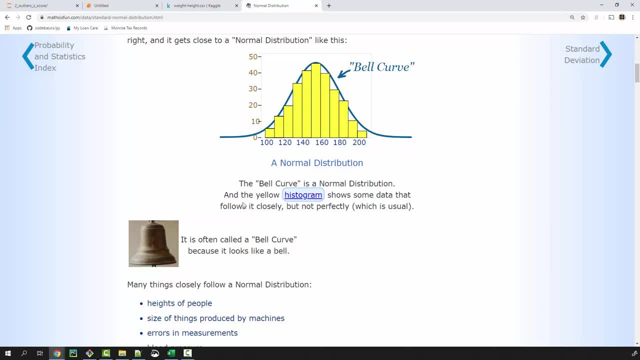 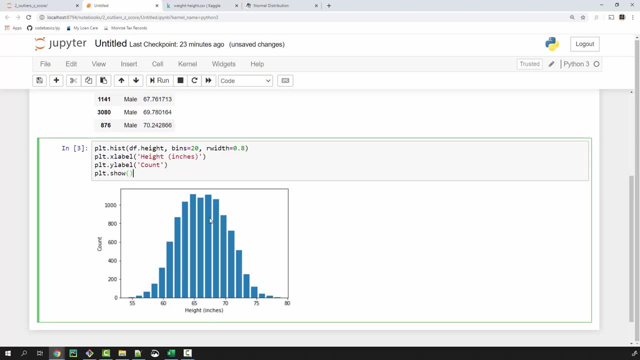 it often has this shape of a bell curve because it looks like a bell and what it means is majority of the values are centered around mean or an average, and then, as you go away from mean, the number of values goes down in nature. we see many data sets which follow normal distribution for 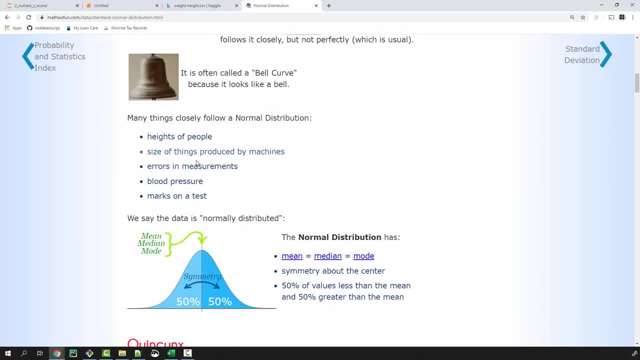 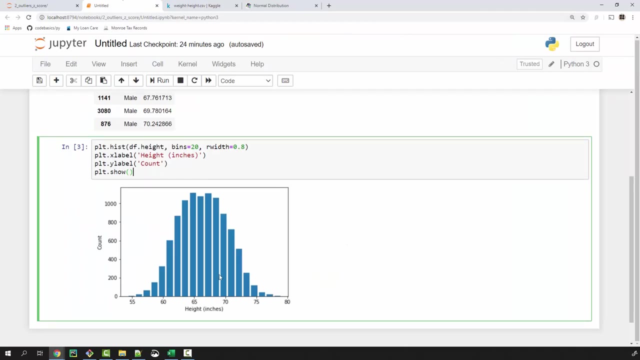 example. here they are saying heights of the people, size of the things produced by machines. you know, blood pressure marks on taste. these are all examples of a normal distribution where, if you are taking example of heights of the people, which is this data set, you will notice that majority of 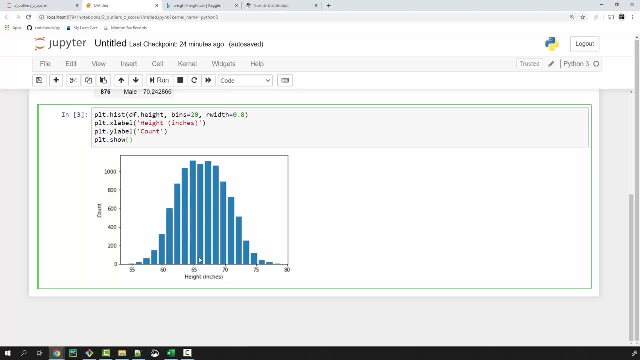 the people have heights between, you know in this area, 65 to 68 inch, and then people having around 80 to 90 inches of height. between the people and the people having around 80 to 90 inches of height, which is more than which is around 7 feet, is very less. so you can see, number of samples are less. 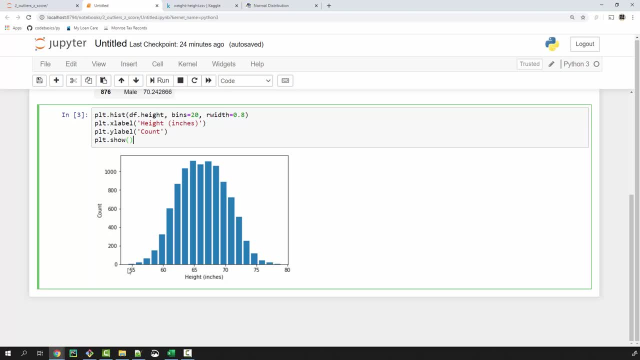 similarly, number of people having very less height, which is like 4 feet, 4 feet, 5 inch, is also less. so this data set is clearly following a normal distribution. now, what we're going to do is we will plot a bell curve that you saw here. so this is: this yellow chart is a histogram, and 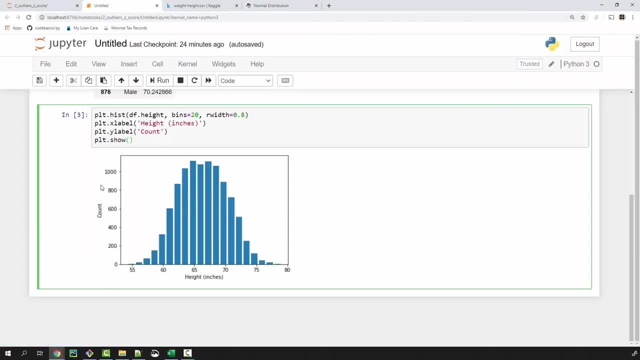 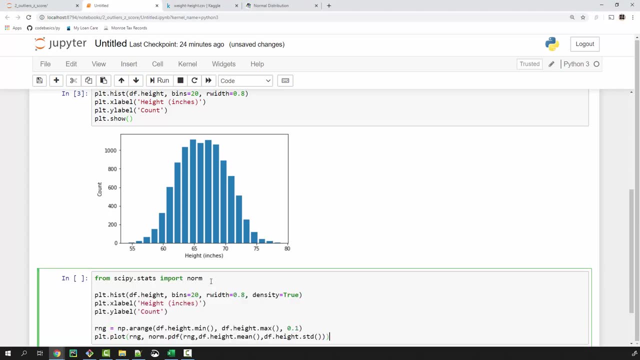 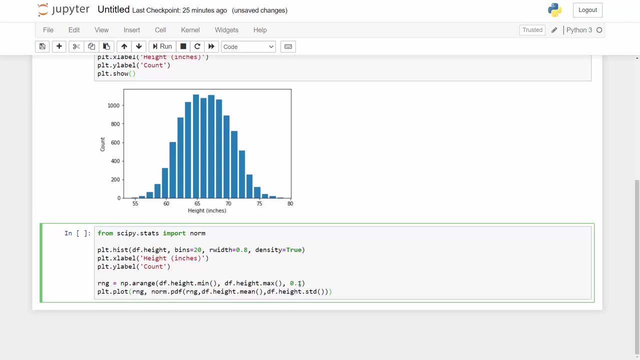 this curve is a bell curl and we'll just plot that bell curve for our visualization purpose, and you will need to use a sci-fi module. so if you have installed sci-fi module already, it, I think, comes with anaconda installation, so you should be good. these three lines are same as this. okay, so you. 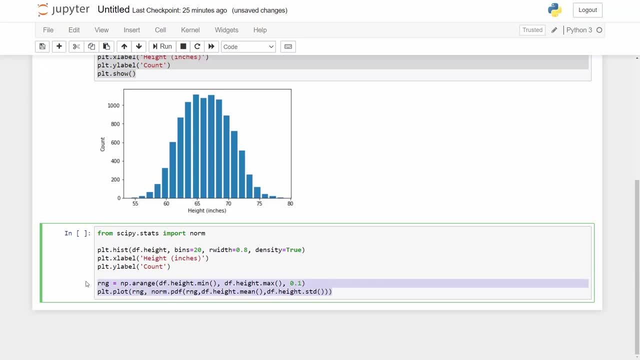 are plotting a histogram here and then, in these two lines, you are plotting the actual bell curve. now we're going to plot a histogram here and then, in these two lines, you are plotting the actual bell curve. now, what are these two lines? so this line is producing the range of x values. so df, dot, height, dot min and. 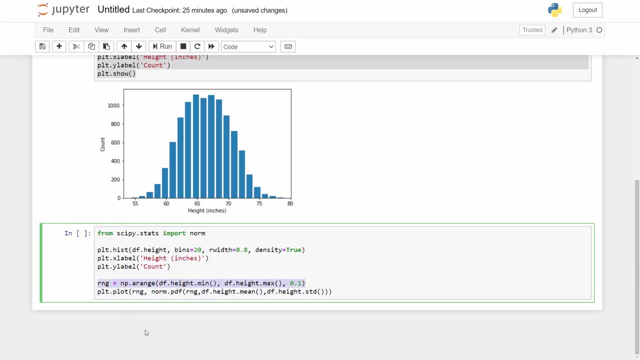 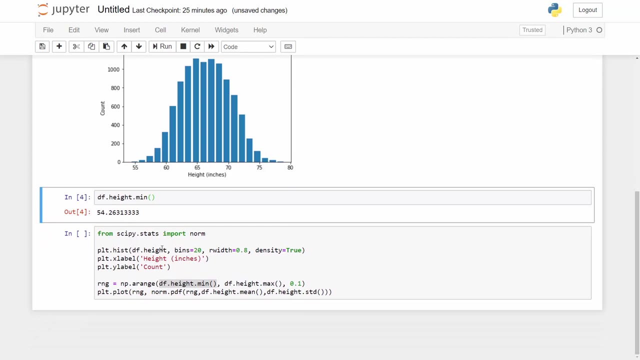 what are these two lines? so this line is producing the range of x values. so df, dot, height, dot, min and max will give you the minimum and maximum value for your height. so let me just print them here for your information. so the minimum height that we see in our data set is 54 inch, which is 4 feet. 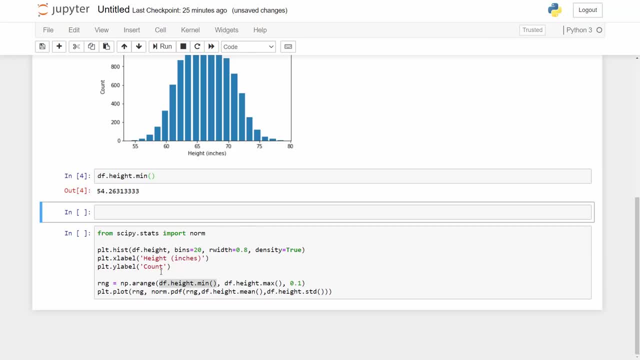 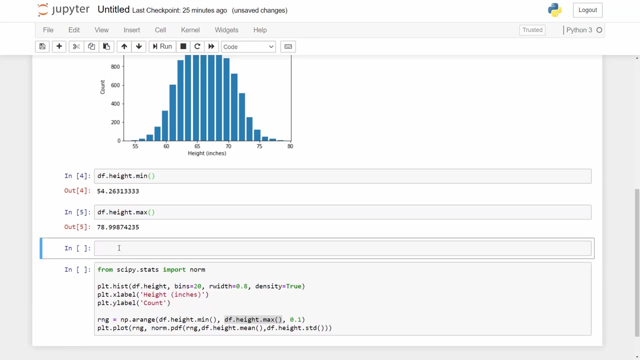 and 6 inch, because 4 feet is 48 inch, so 4 feet and 60 and 6 inch. the max height in the data set is 78 inch, which is around 6 feet 6 inch. okay, you can also do describe and that will tell you. 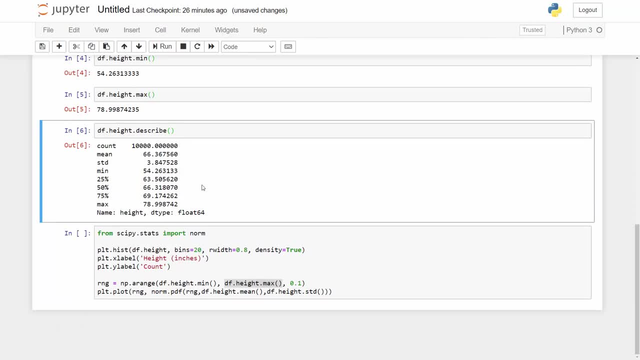 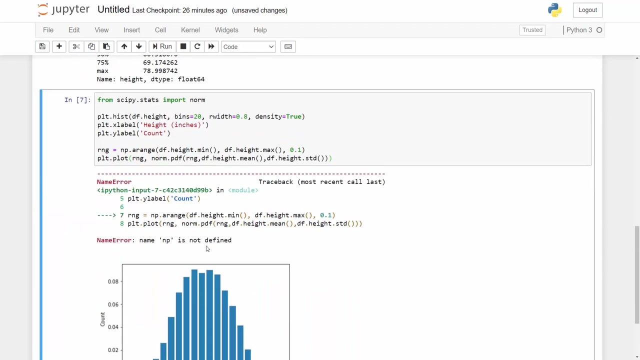 the quick statistics on the height column, you know. here it says minimum height is 54, max is 78. then this is a standard deviation. the count is 10 000. we saw excel file has 10 000 data points. okay, uh. so once this is all done, you can now execute this cell and it will plot the uh chart for you. 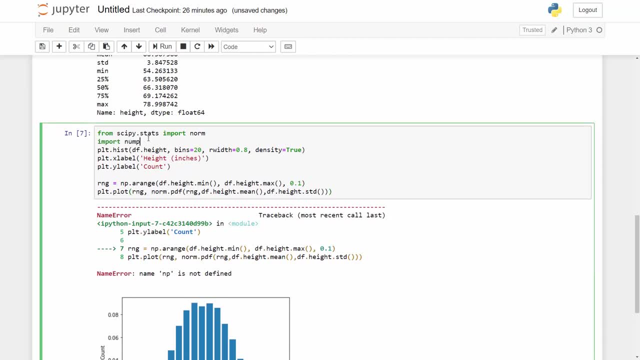 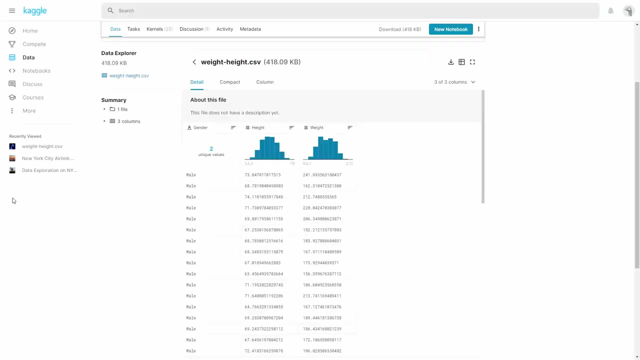 now, np is not defined here, so i will say import numpy as np and that will plot this nice looking bell curve for you. and this bell curve clearly shows normal distribution. uh, we already saw on this particular chart, you know. if you remember this chart, see, it shows the normal distribution here. 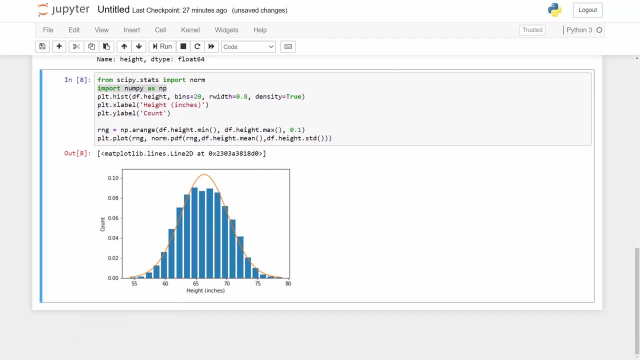 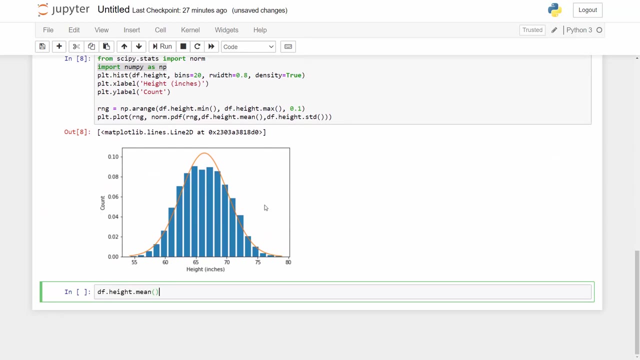 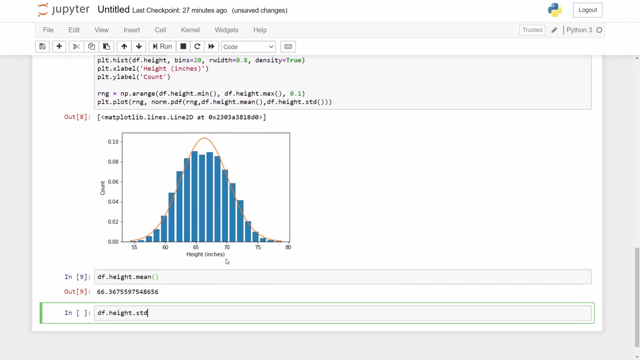 now what we're going to do next is find out the mean and standard deviation. now, mean and standard deviation we already saw in this describe parameter. but if you want to just kind of print it out, then you can say: df dot height, dot, mean. that will print the mean of this column, and then df dot height, dot, std. this. 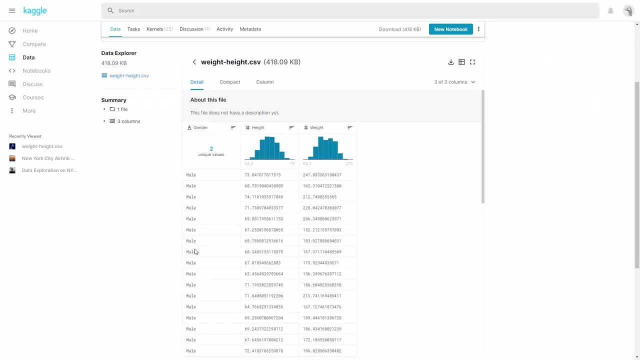 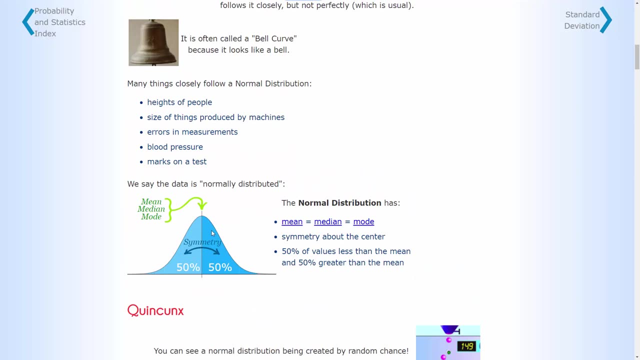 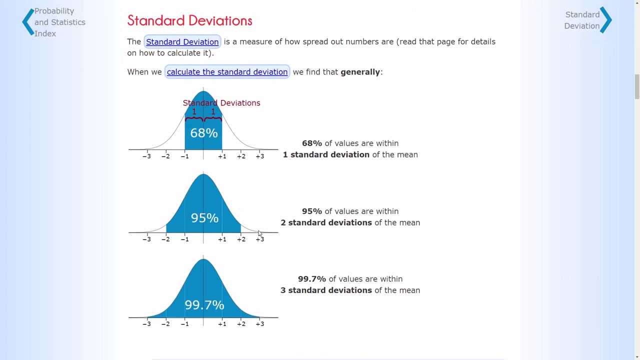 is printing standard deviation. now, what is standard deviation if you don't know? standard deviation is basically showing you how far away the data point is from mean value. okay, so, uh, in this example, most of the data points are within one standard deviation. if your data set is uh, normally. 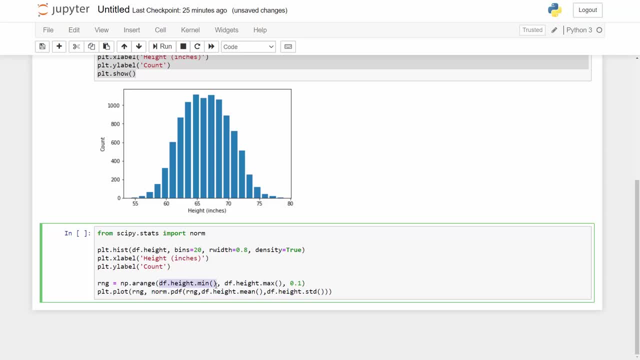 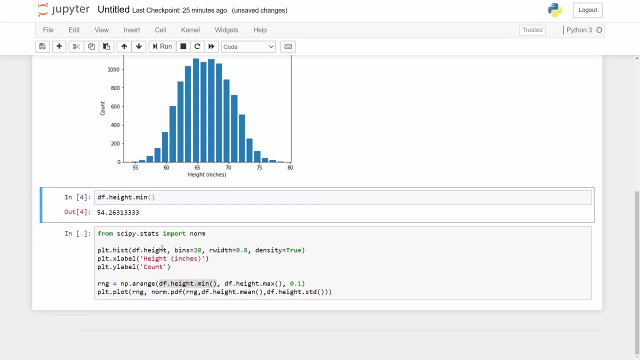 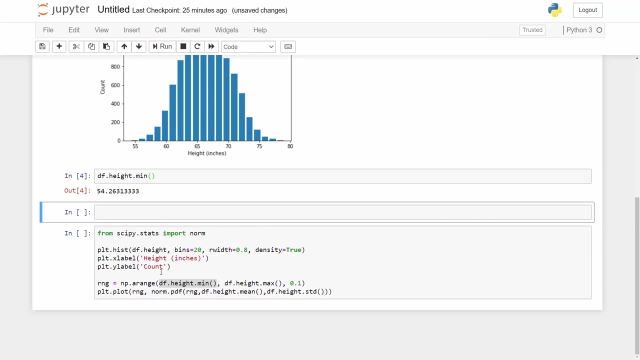 max will give you the minimum and maximum value for your height. so let me just print them here for your information. so the minimum height that we see in our data set is 54 inch, which is 4 feet and 6 inch, because 4 feet is 48 inch, so 4 feet and 60 and. 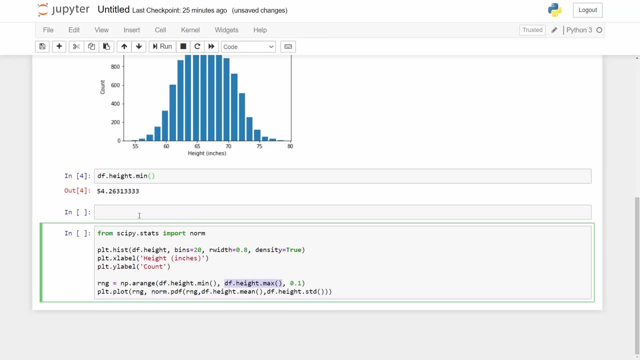 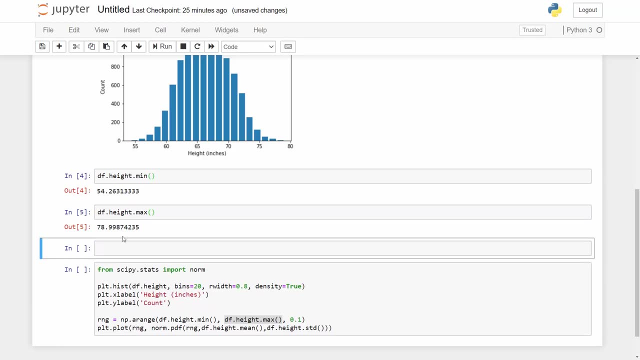 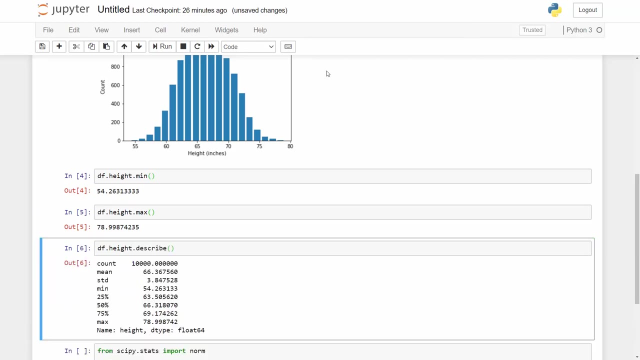 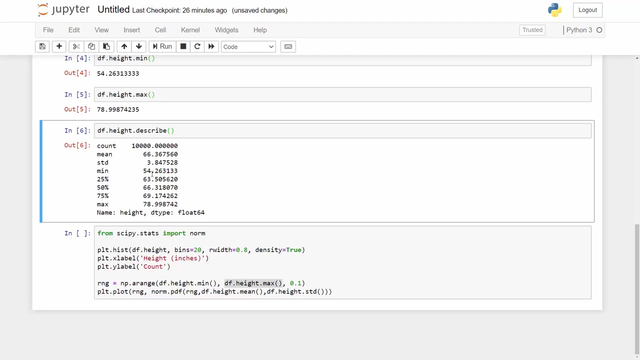 6 inch. the max height in the data set is 78 inch, which is around 6 feet 6 inch. okay, you can also do describe and that will tell you the quick statistics on the height column. you know, here it says minimum height is 54, max is 78. then this is a 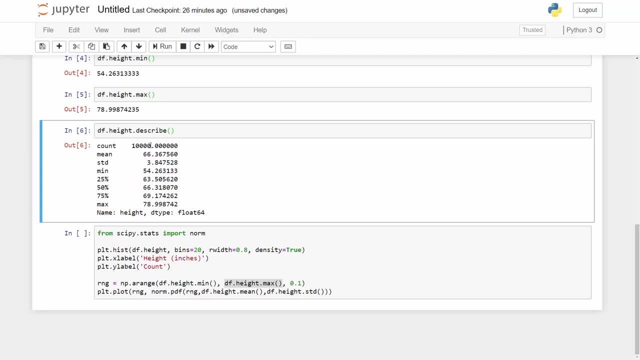 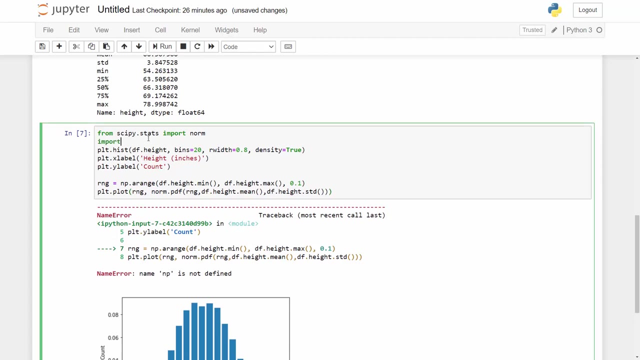 under deviation, the count is ten thousand. we saw excel file has ten thousand data points. okay, uh. so once this is all done, you can now execute this cell and it will plot the uh chart for you. now, np is not defined here, so i will say import numpy as np, and that will. 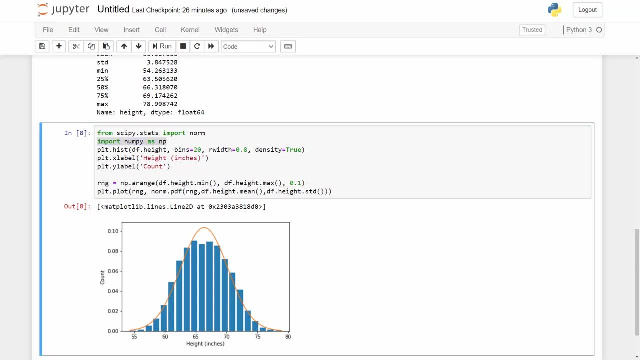 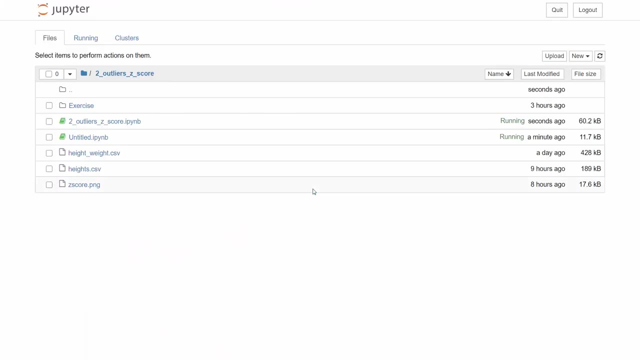 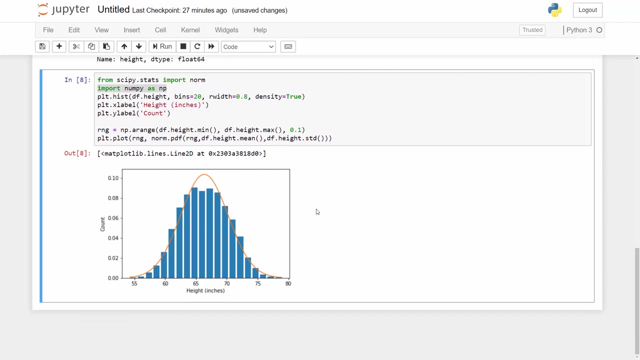 plot this nice looking bell curve for you, and this bell curve clearly shows normal distribution. uh, we already saw on this particular chart, you know. if you remember this chart, see, it shows the normal distribution here. now, what we're going to do next is find out the mean and standard. 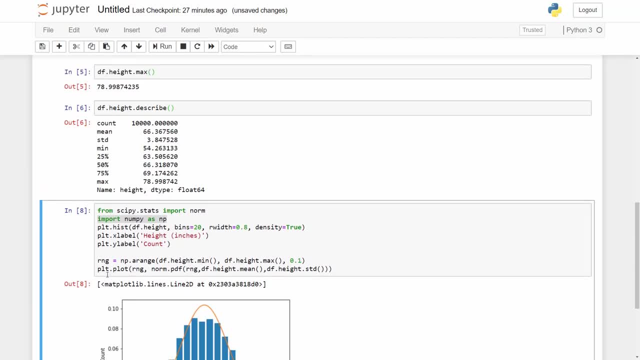 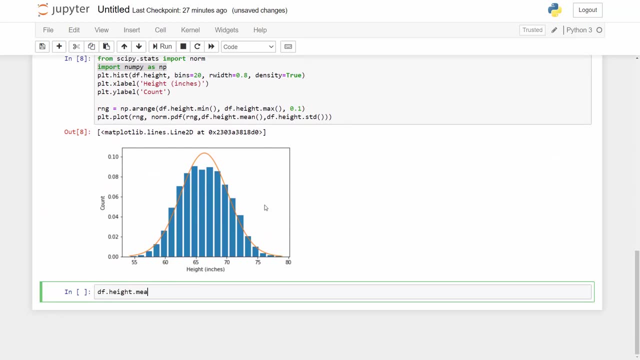 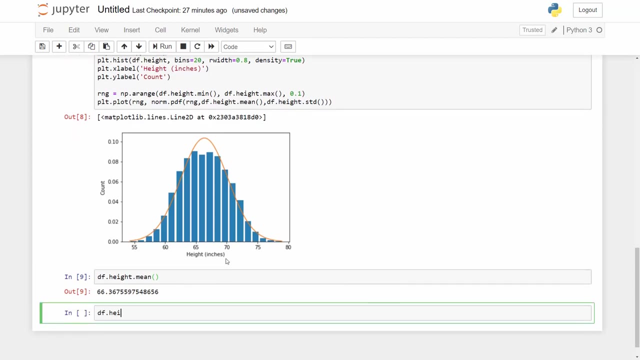 deviation now mean, and standard deviation we already saw in this describe parameter. but if you want to just kind of print it out, then you can say: df dot, height, dot mean. that will print the mean of this column, and then df dot height, dot, std. this is printing standard deviation now. 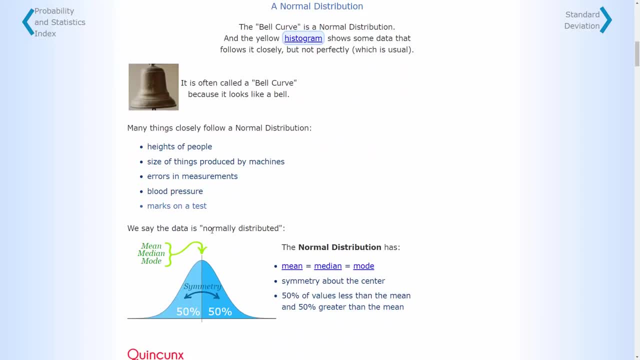 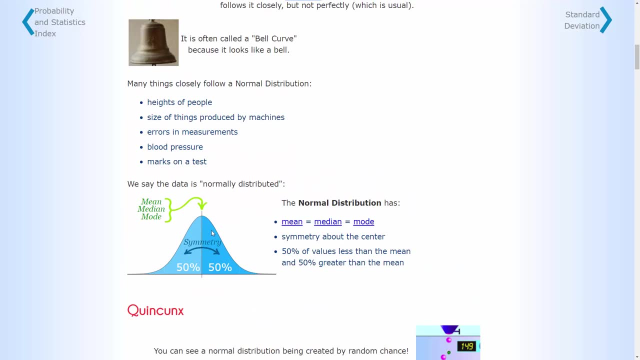 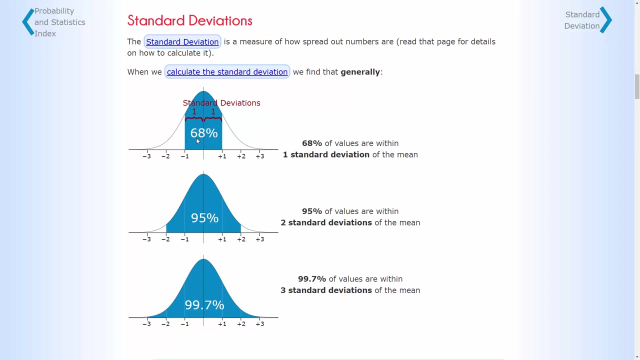 what is standard deviation if you don't know? standard deviation is basically showing you how far away the data point is from mean value. okay, so in this example, most of the data points are within one standard deviation. if your data set is normally distributed, 68 percent of the samples will be within one. 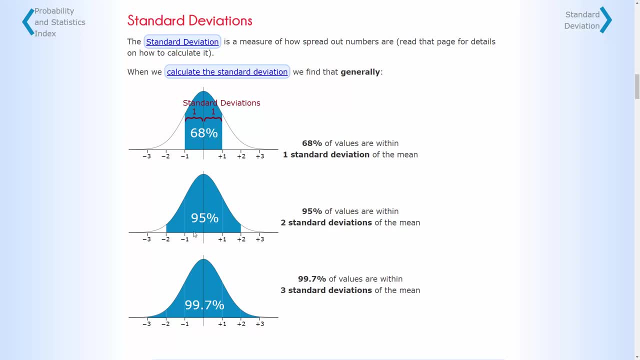 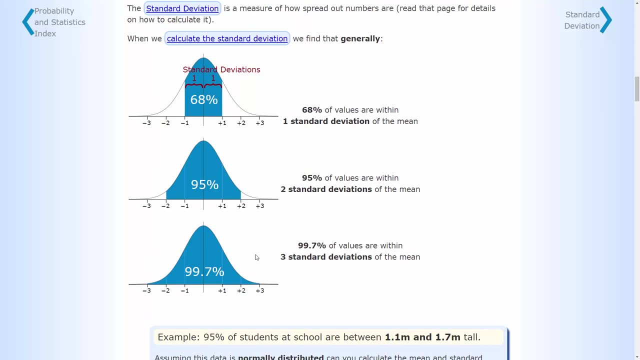 standard deviation value, then 95 percent samples will be in two standard deviation and 99.7 percent samples will be in three standard deviation. okay, uh, so standard deviation is just, it's nothing, but it just shows you how far away you are from mean. for example, our mean value is 66 inch. 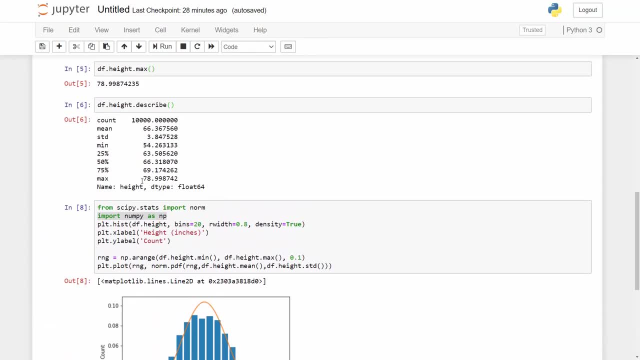 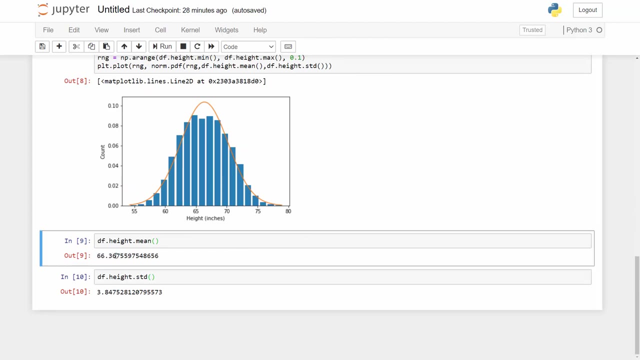 and if we have a data point which is, let's say this one, 78, so 78 is quite far away from your max, so this will naturally have a higher standard deviation. but if you have something like, let's say, 67, 68, then those will be most likely within one standard. 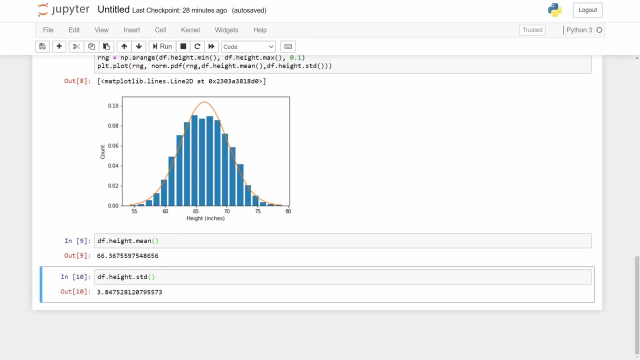 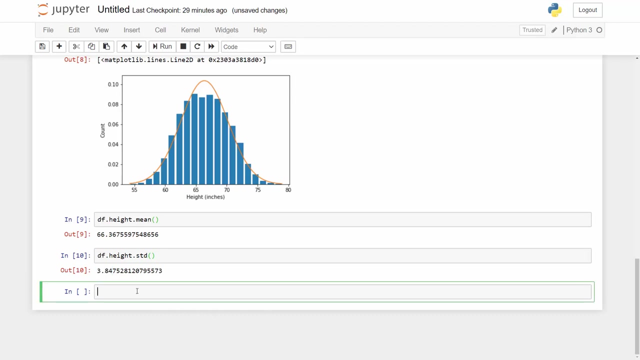 deviation range. so see what this shows is if you have anything in like 3.84 range from 66. so 66 plus 3.84 is one standard deviation away. minus 3.84 is two standard deviation away. so now we will use three standard deviation first to remove the outliers. so three standard deviation is kind. 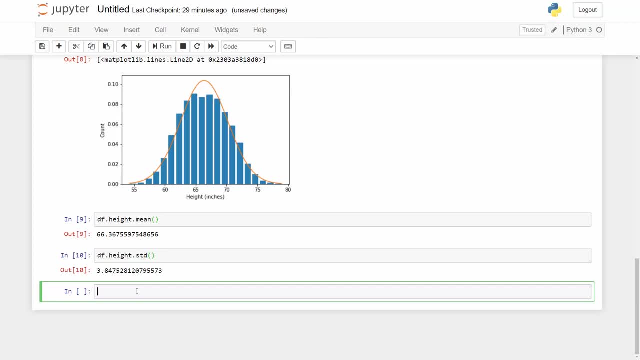 of a common practice in the industry to remove the outliers. sometimes people use four standard deviation, five standard deviation as well if the data set is small. I have seen people using even two standard deviation. but you have to really use the sense of your judgment to come up with 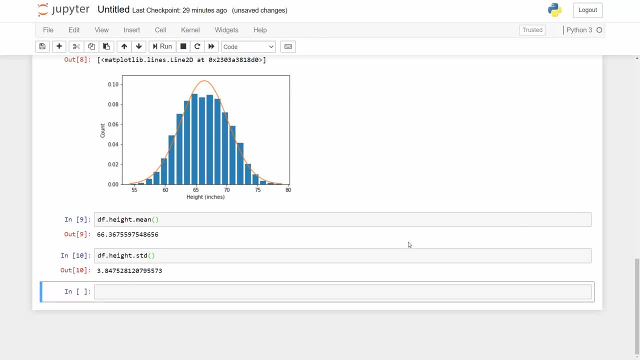 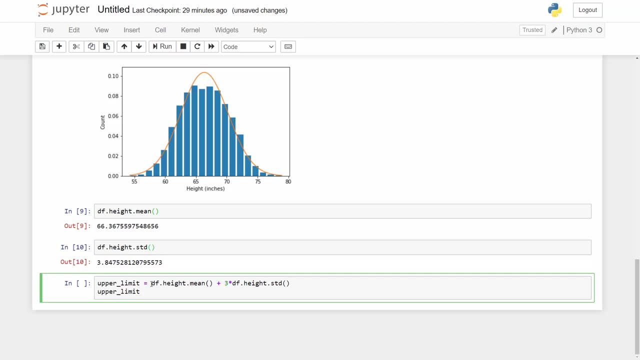 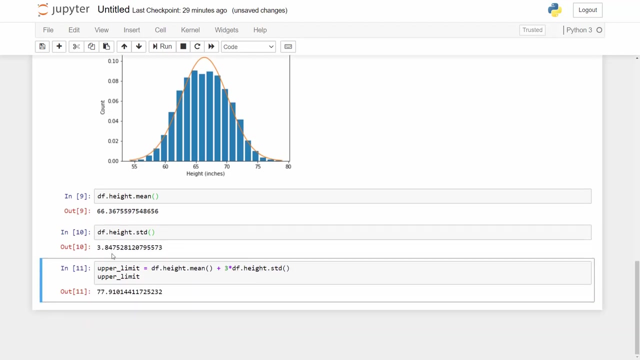 that threshold on how many standard deviations are there you want to use. so here I will figure out my upper limit by saying: okay, I want mean and three standard deviation to be my upper limit, and anything which is more than 77.91 I'm gonna. 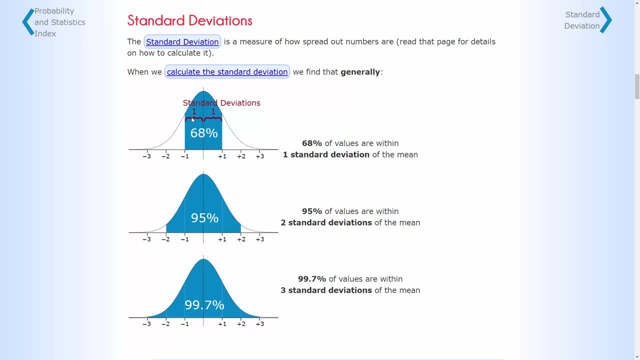 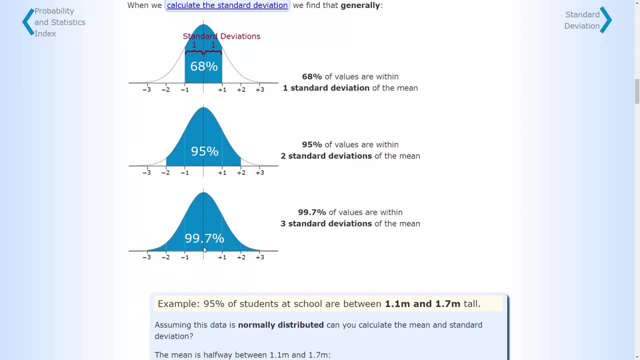 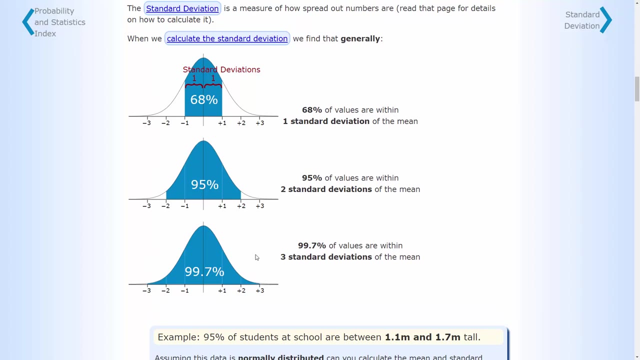 distributed, 68 percent of the samples will be within one standard deviation value, then 95 samples will be in two standard deviation and 99.7 percent samples will be in three standard deviation. okay, uh, so standard deviation is just, it's nothing, but it just shows you how far away. 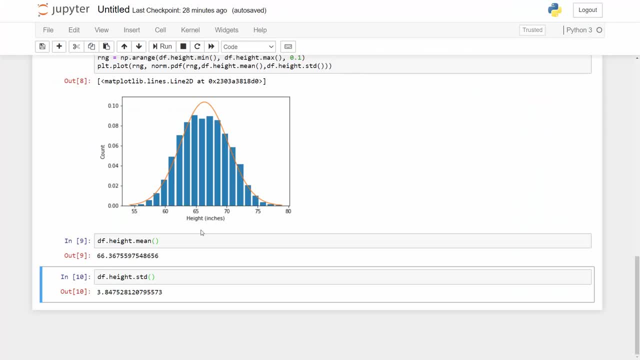 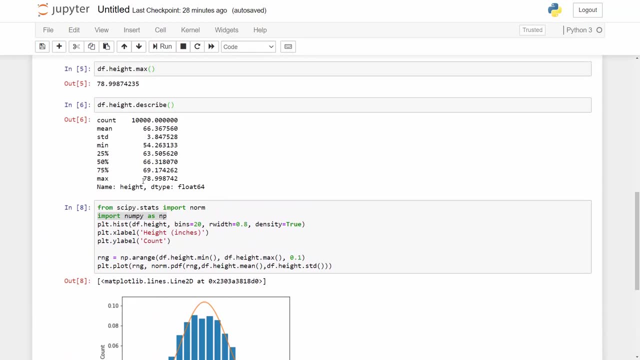 you are from mean. for example, our mean value is 66 inch and if we have a data point which is, let's say this one, 78. so 78 is quite far away from your max, so this will naturally have a higher standard deviation. but if you have something like, let's say, 67, 68, then those will be most likely within 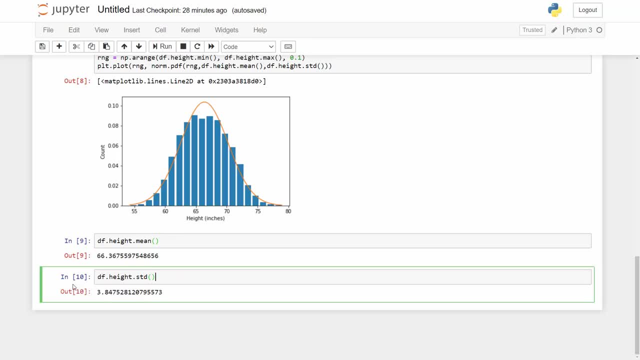 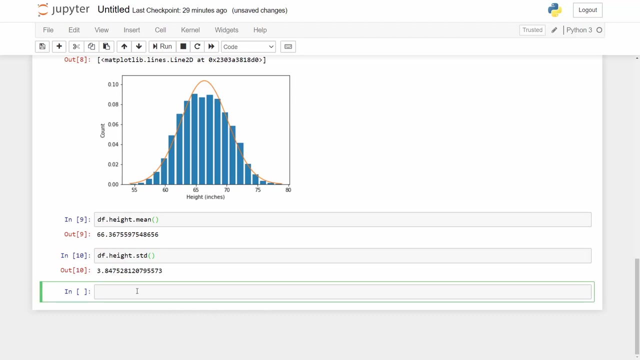 one standard deviation range. so see what this shows is if you have anything in like a 3.84 range from 66. so 66 plus 3.84 is one standard deviation away, minus 3.84 is two standard deviation away. so now we will use uh three standard deviation first to remove the 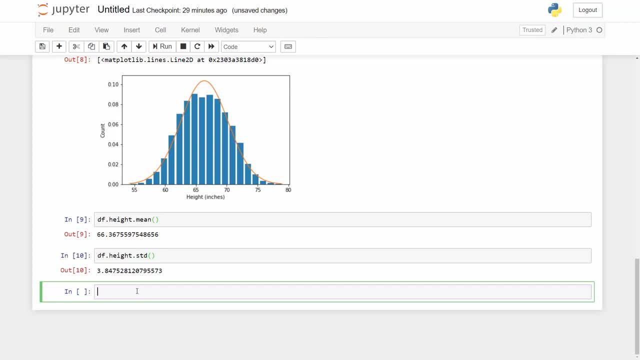 outliers. so three standard deviation is kind of a common practice in the industry to remove the outliers. sometimes people use four standard deviations and five standard deviation as well. if the data set is small i have seen people using even two standard deviation. but you have to really use the sense of your judgment, uh, to come up with 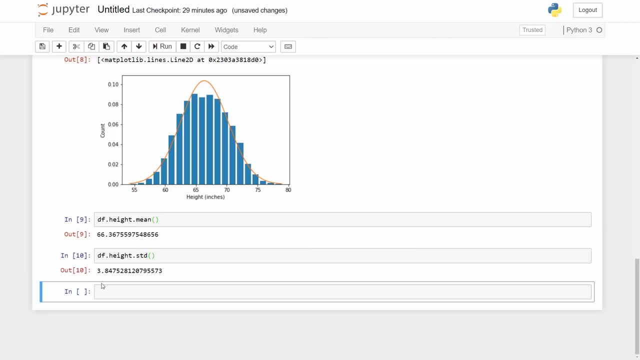 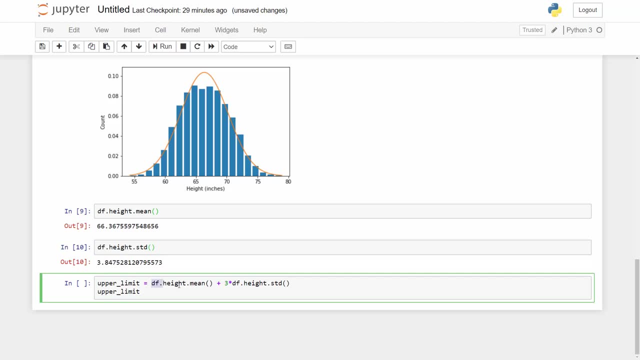 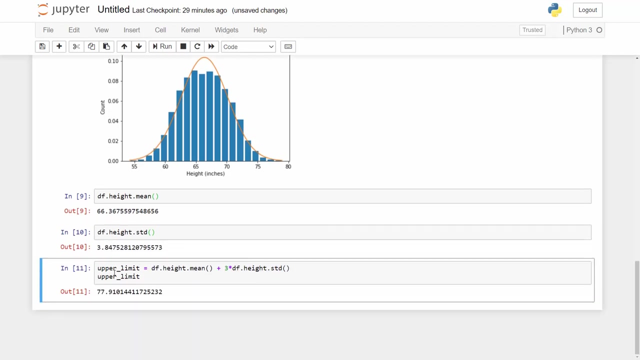 that threshold on how many standard deviation you want to use. so here, uh, i will figure out my upper limit by saying: okay, i want mean and three standard deviation to be my upper limit and anything which is more than 77.91. i'm gonna mark that as an outlier. 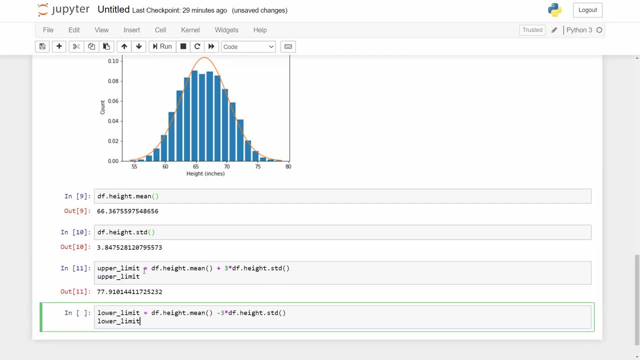 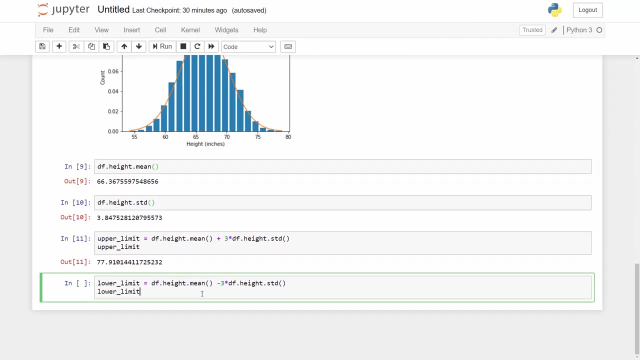 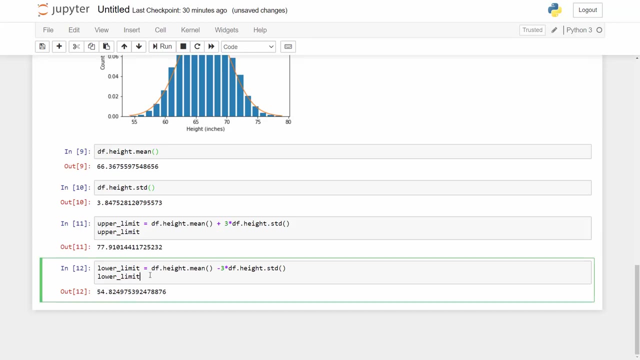 you can do similar thing on lower end and you can say: mean height minus 3 standard deviation is my lower limit, which means any height less than 54.82. i will mark that as an outlier. now let's quickly see what are the outliers in the standard deviation range. so let's look at the outliers in the 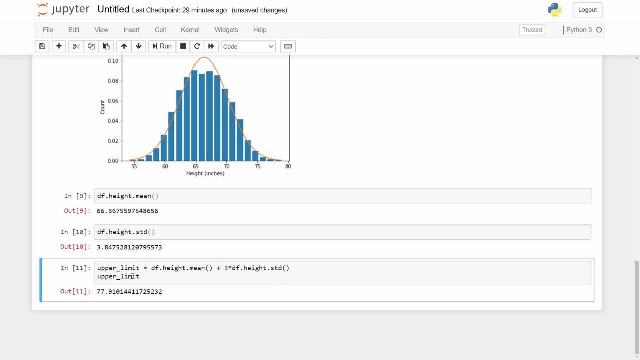 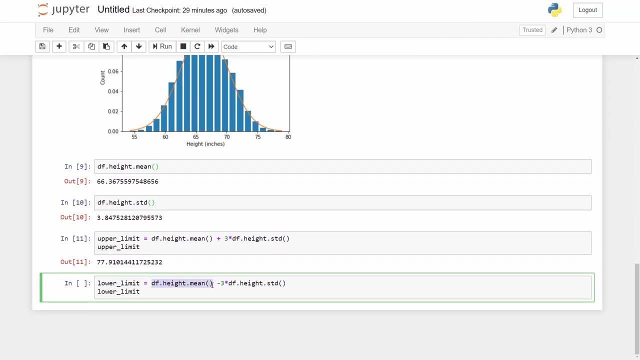 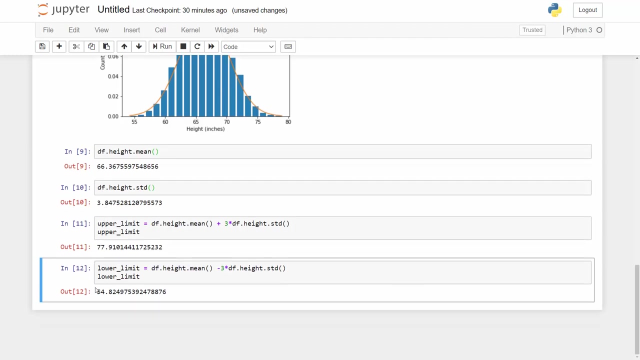 mark that as an outlier. you can do similar thing on lower end and you can say: mean height minus three. standard deviation is my lower limit, which means any height less than 54.82. I will mark that as an outlier. now let's quickly see what are the outliers in our data frame. so in our data frame, 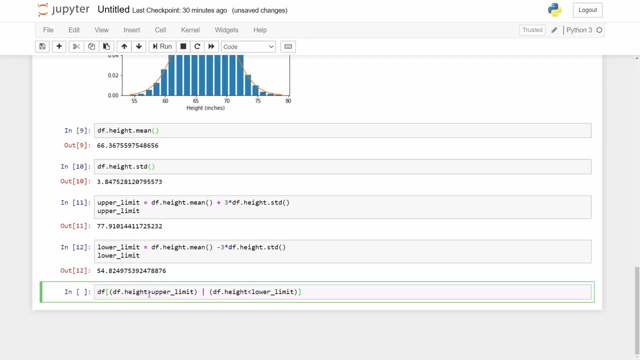 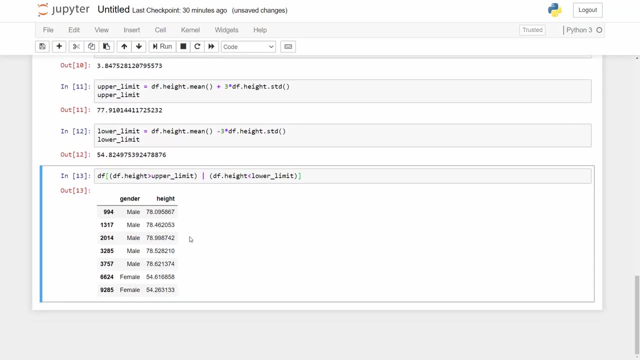 when you do something like this, where you're saying if my height is greater than upper limit or lower than lower limit, then show me those data points. and I find this only at the center of that area, which is 72.keepers. so then say at the center of that area. 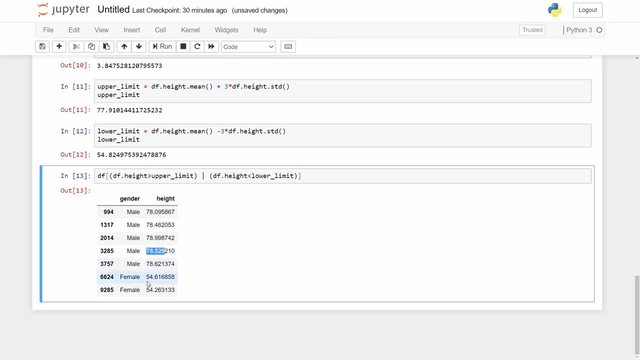 where I need to make sure our platform is. Feel free to pick the outliersyang of my journey where ways i can convert that data that way and also when we like to have some kind of outlier, Конечно, can be different. if it's more regular, you not of interest, it's another. 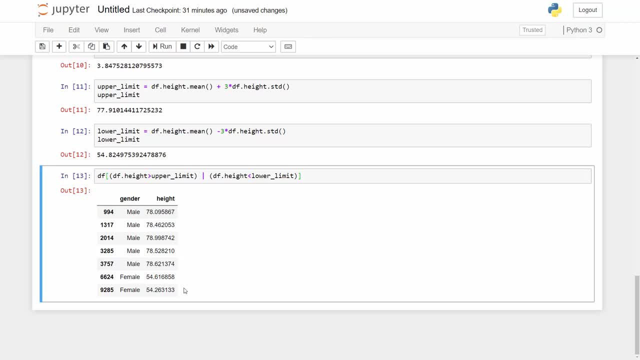 one function too, and another is just expression. If we want to make sure high speed, extremely short space for even a pilotsome, so that just hurt you saying: and всей measures from every in none at anything particularly will. can we do different agent without? when limit we activity, it'll trickle down. but see where the data point is. 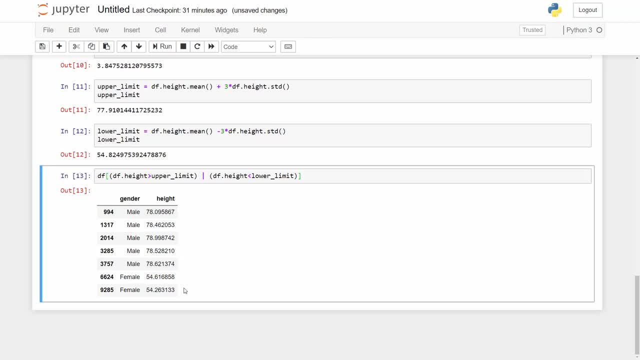 Can actually remove those points as an outlier because that can help With your model or it can generally help with your data analysis process. Sometimes the big because of the error, you might see crazy values such as you know. you might see, let's say, 2,000 or 1,000, those kind of crazy values. 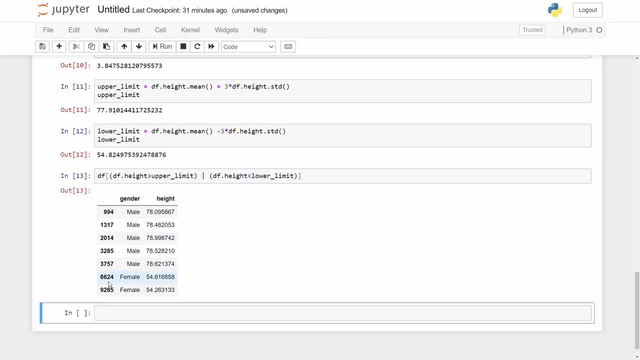 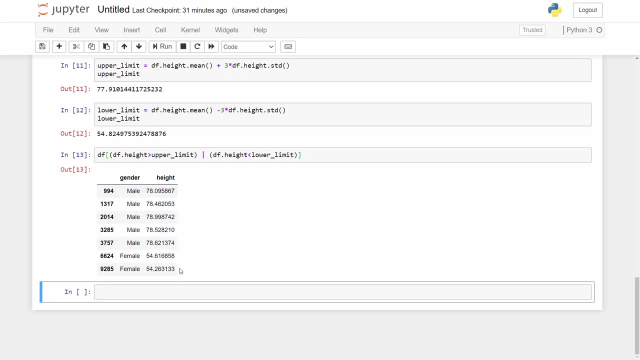 In that case, removing those outlier becomes really easy. You don't have to think much. but here you know, I can discuss this result with my business manager, for whom I'm building my model, and If he agrees, I can remove these as an outlier. Okay, and how do you remove these as an outlier? So 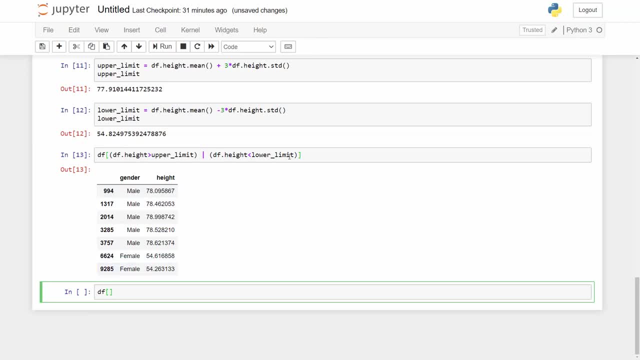 What you can do is you can say DF Okay, and here you can specify a condition. so you you can say DF dot height. I want the height to be in this limit. It should be less than upper limit and the height should be greater than. 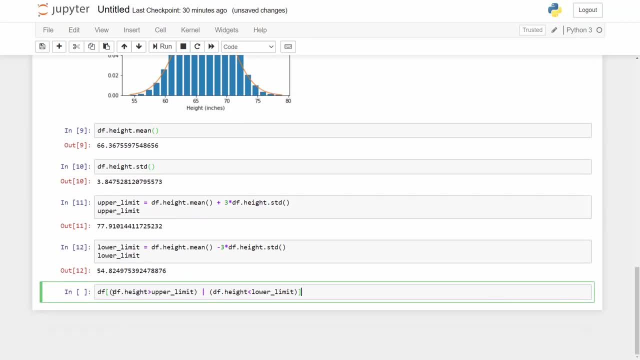 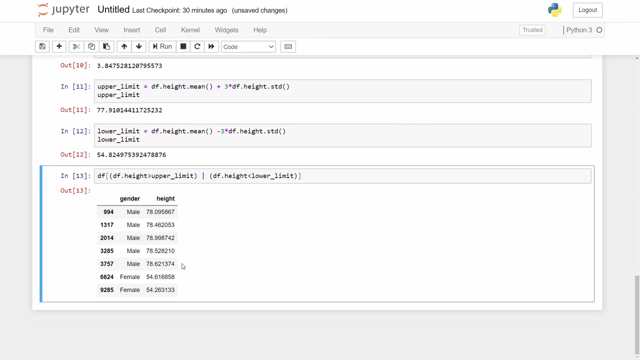 in our data frame. so in our data frame, when you do something like this where you're saying if my height is greater than upper limit or lower than lower limit, then show me those data points, and I find this seven data points where the height is really high. this is six four, six feet six inch. actually the height is 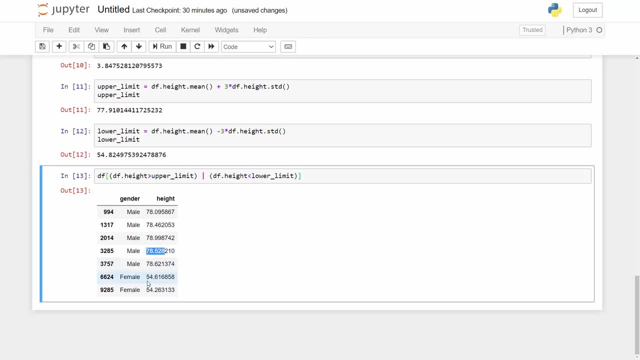 an inch you can convert it into feet. an inch 54 is four feet six inch. now these heights are actually- they might be- valid heights. you know, I'm not saying these are data errors, but many times, even if the data point is legitimate, we can actually remove those points as an outlier, because that can help with your. 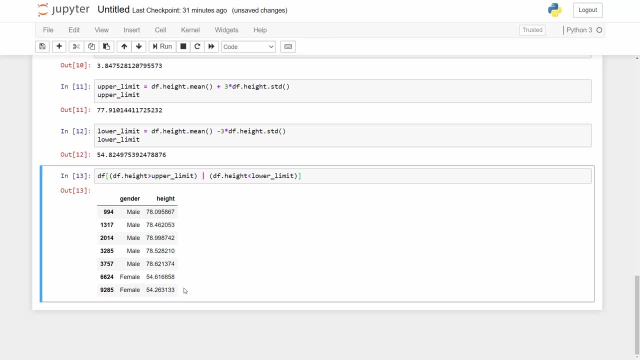 model or your data frame. so if you want to convert it into feet an inch, you can general help with your data analysis process. sometimes the because of the error, you might see crazy values such as you know. you might see, let's say, 2000 or 1000, those kind of crazy values. in that case removing those outlier becomes. 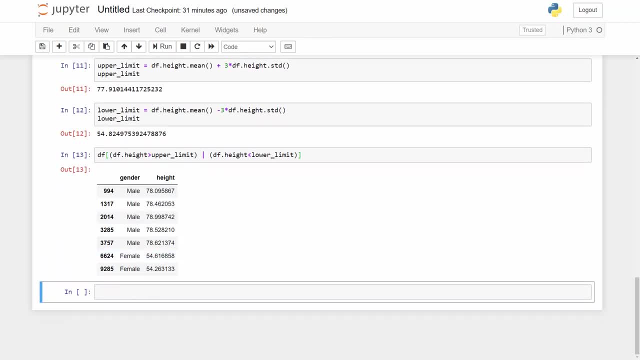 really easy. you don't have to think much. but here you know, I can discuss this result with my business manager, for whom I am building my model, and if he agrees, I can remove those feet andficiente値maredness weights~~. the data points, wouldrikers and weights, are similar in size and each of them 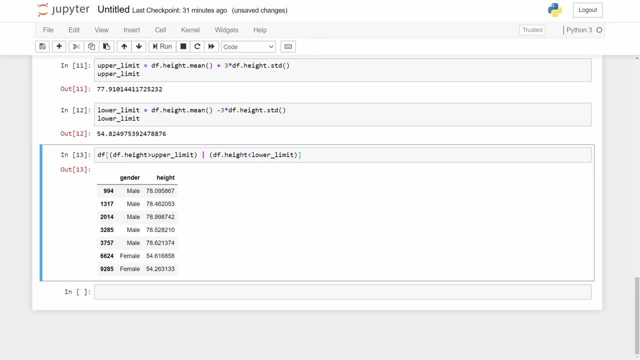 would find- and speak in their own language in the actual lookup that it does- that these as an outlier okay, and how do you remove these as an outlier? so what you can do is you can say DF okay, and here you can specify a condition, so you, you. 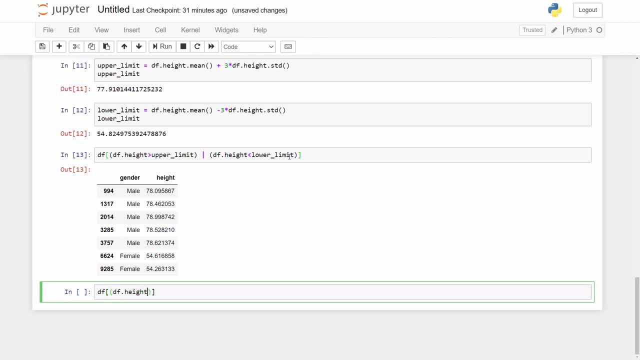 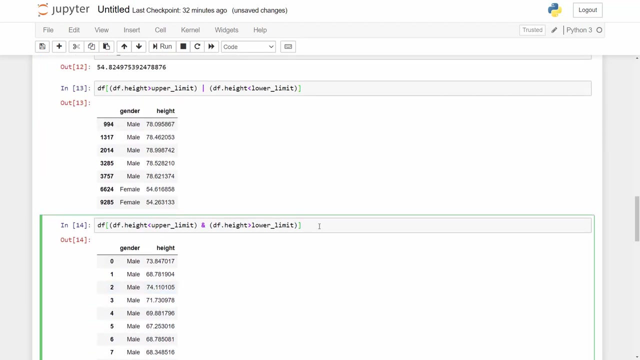 can say DF dot height- I want the height to be in this limit- it should be less than upper limit and the height should be greater than lower limit- and say it will give you this data frame which will have your normal, like good-looking data points. okay, and this you can store in a new data frame and this new data frame. 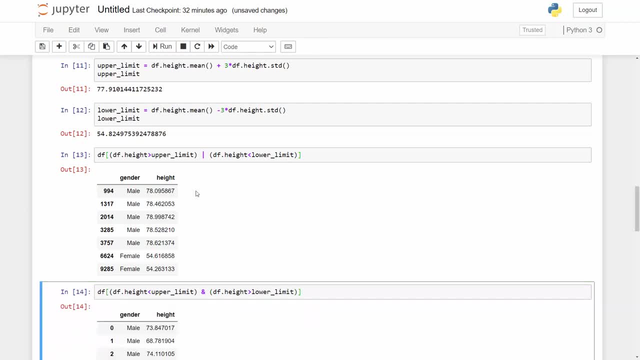 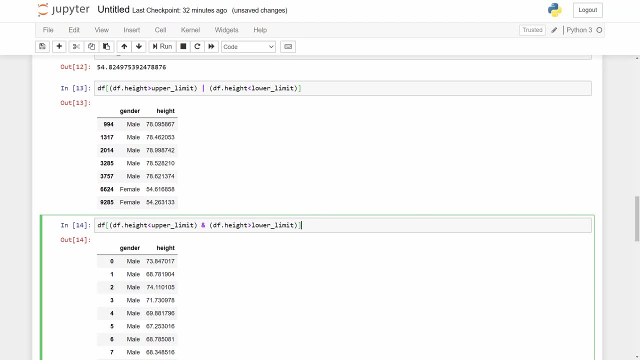 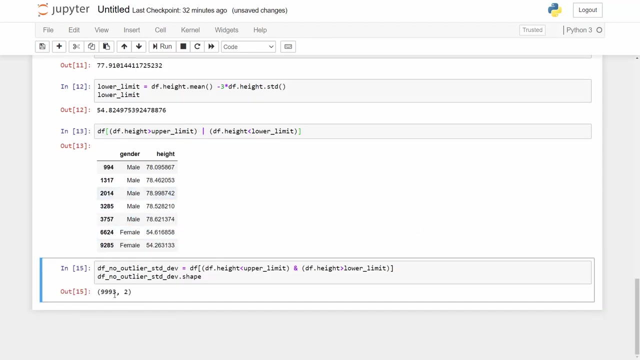 lower limit and Say it will give you this data frame which will have your Normal, like good-looking data points. Okay, and this you can store in a new data frame. and This new data frame, you can just print a shape of it And you will find that, out of ten thousand nine hundred nine thousand nine nine three are the valid samples. 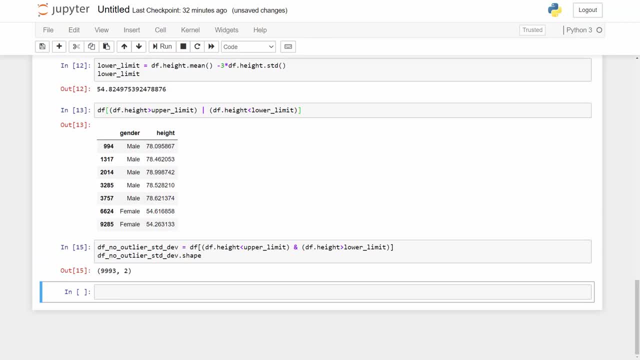 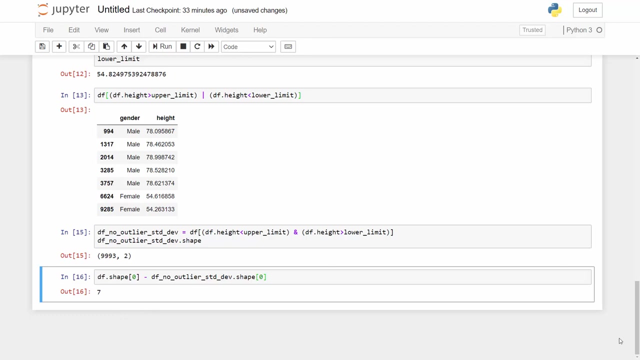 Okay, so you can just say: This is the shape of your filtered out data frame and if you do, Shape of zero will return your number of rows. Okay, and if you do this, you will find that you removed seven outliers using this method. Now we are going to use z-score to do the same thing. now z-score and standard deviation are kind of very similar things. 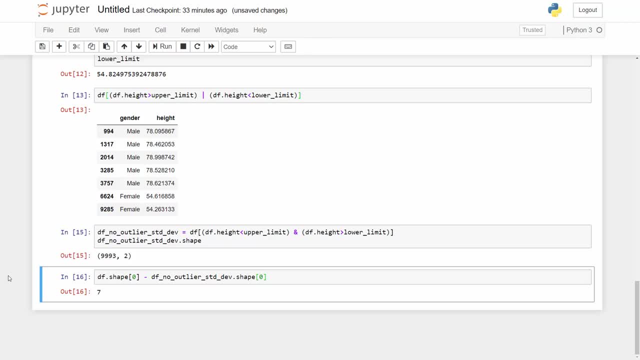 Z-score just tells you the. it gives you a number which will tell you how many standard deviation you are away from the mean. so let's say, if your data point is three standard deviation away, then the z-score for that data point will be Three. if it is two point five standard deviation away, then it will be two point five. 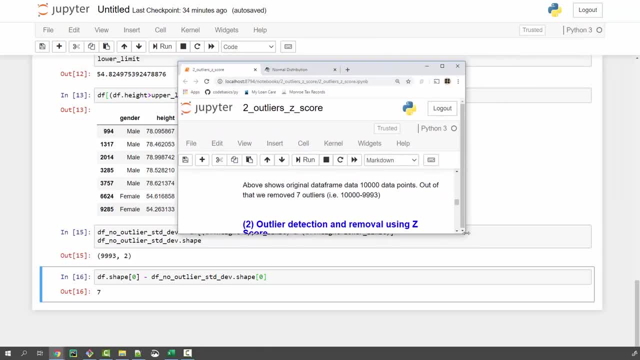 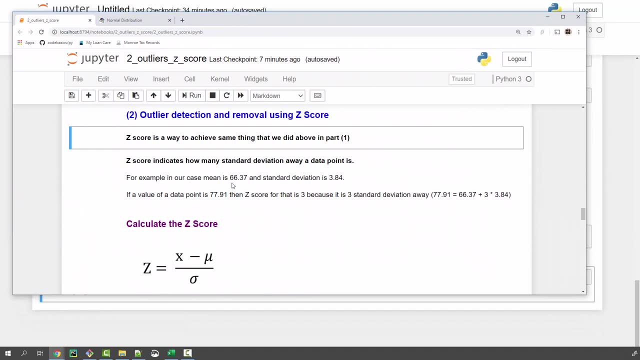 Okay, So I'm just gonna pull this other notebook and just kind of walk you through the definition of z-score and the equation. So see, here it's saying it indicates how many standard deviation away your data point is. for example, our mean is sixty six point three seven and three point eighty four is the. 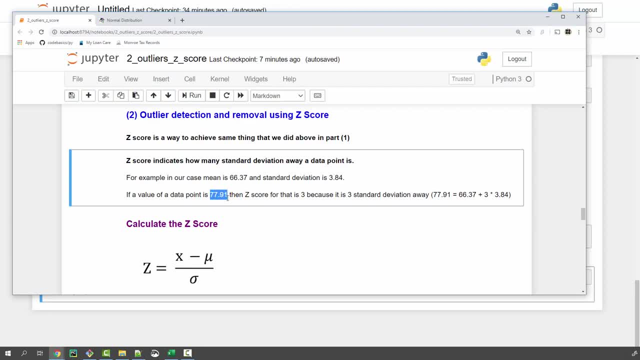 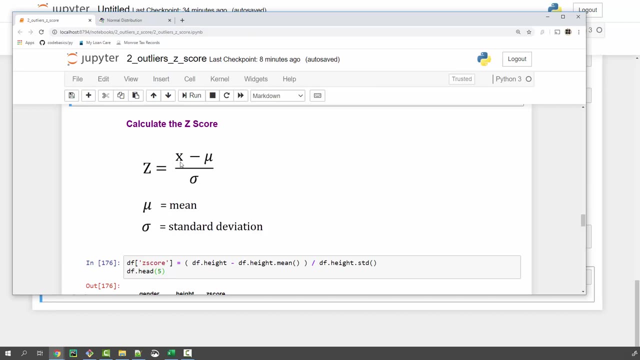 standard deviation, and if your data point is seventy seven point ninety one, then the z-score will be three, because Seventy seven point ninety one is three standard deviation away. The equation is extremely simple: The z-score is equal to ux, which is your data point value, which in this case was seventy seven point ninety one. 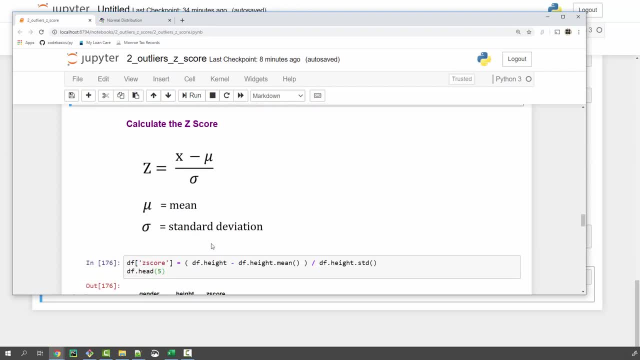 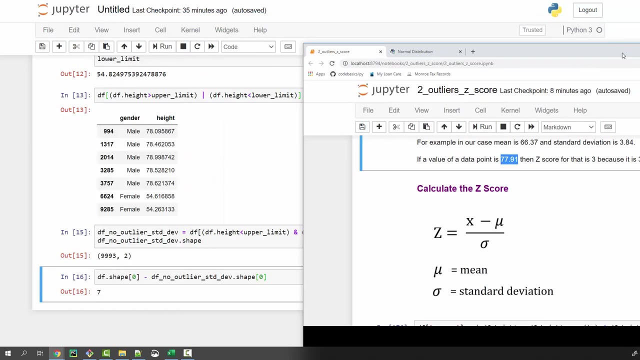 minus mean Divided by standard deviation. Okay, So this is an extremely simple equation. z-score is extremely simple thing, guys like, don't this? There is not no rocket science in it. It is Very similar to standard deviation: It just tells you a number on how many standard deviation you are away from the mean. and 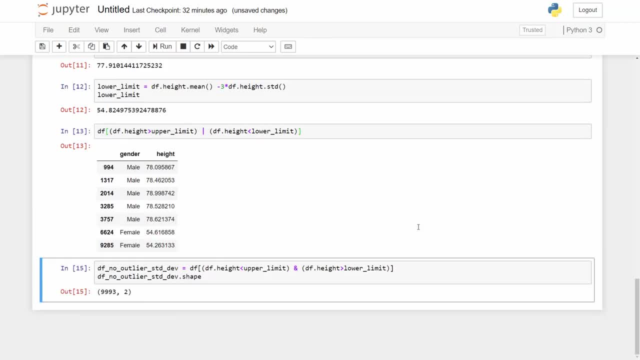 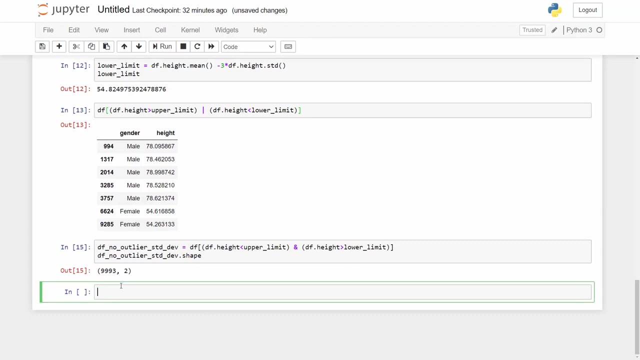 you can just print a shape of it and you will find that, out of ten thousand nine hundred nine thousand nine nine three are the valid samples. okay, so you can just say this is the shape of your filtered out data frame and if you do, shape of zero, will return your number. 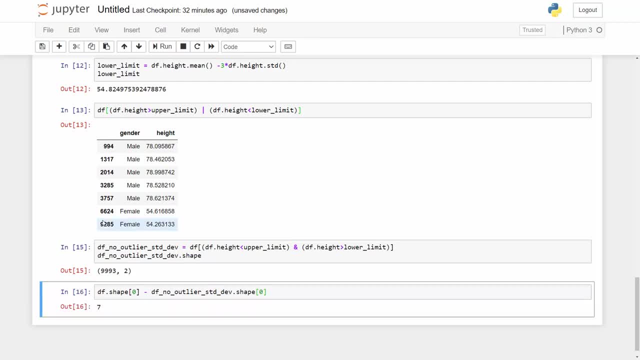 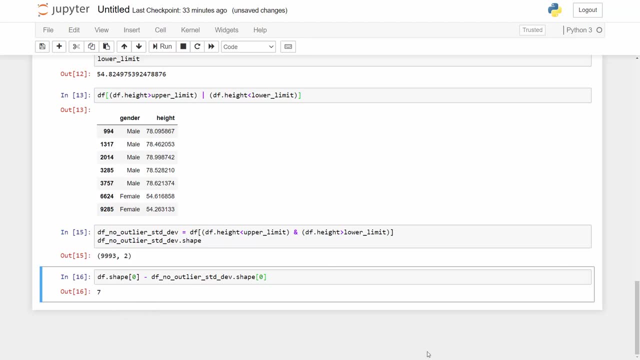 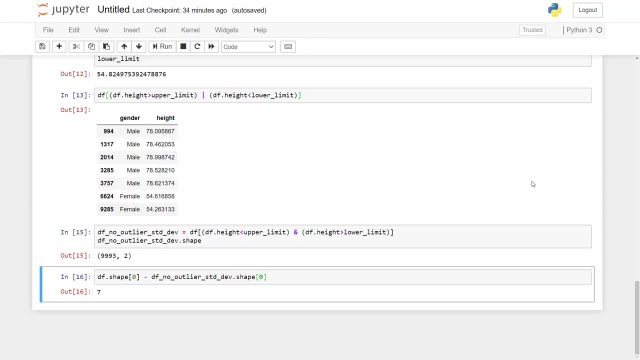 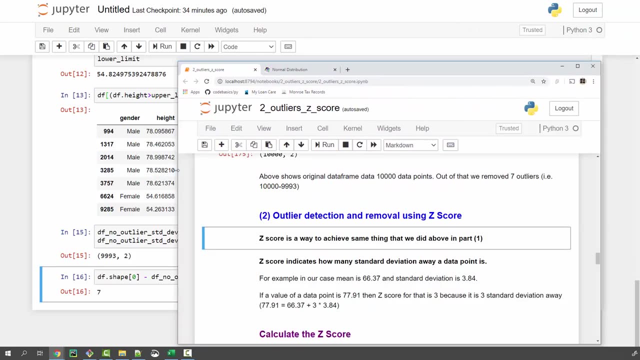 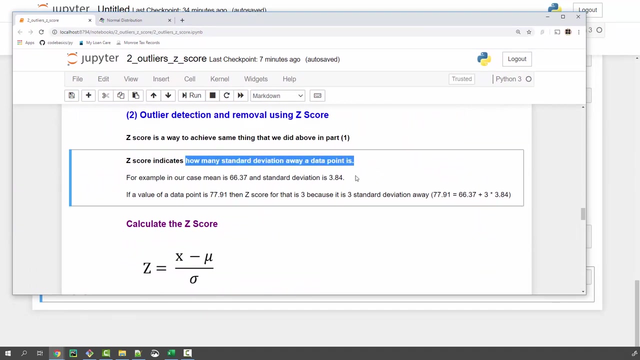 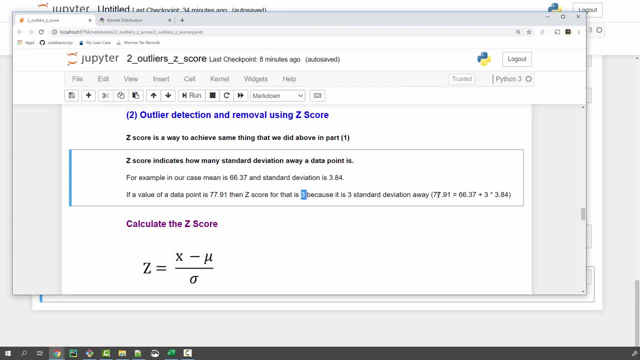 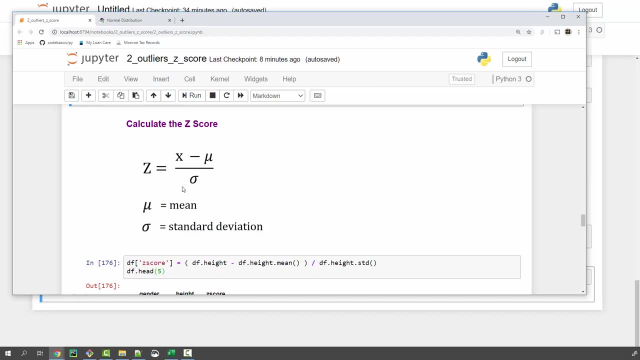 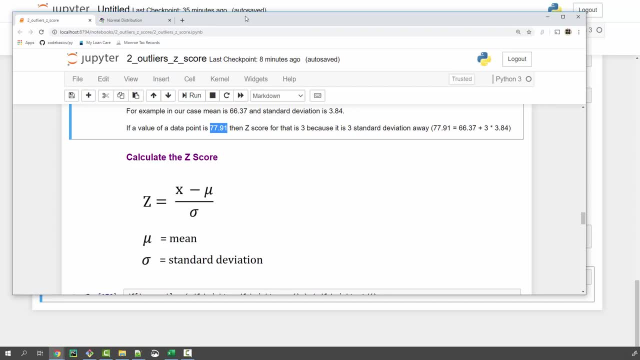 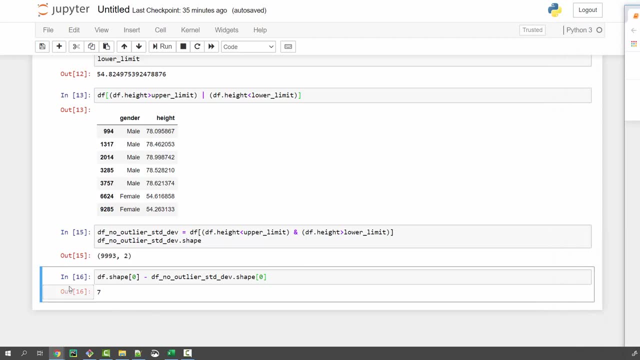 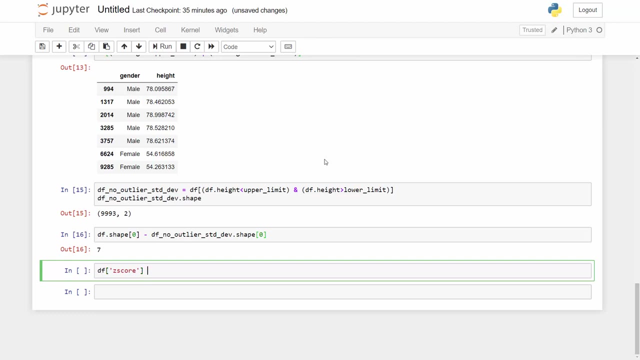 in it. it is very similar to standard deviation. it just tells you a number on how many standard deviation you are away from the mean. and to calculate the z score, i'm going to create a new column in my data frame. call it z score, and you might know that this is how you can create new. 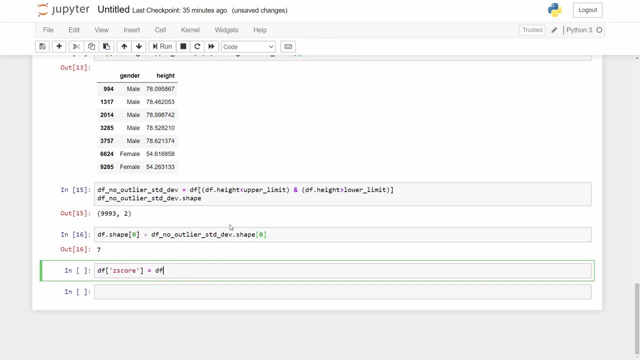 columns in the data frame. okay, and this will be dependent on my height minus height mean. okay, so it's like x which is your, this data point minus mean, divided by the standard deviation. and this is how you can get standard deviation: df dot height gives you a column in the data frame. 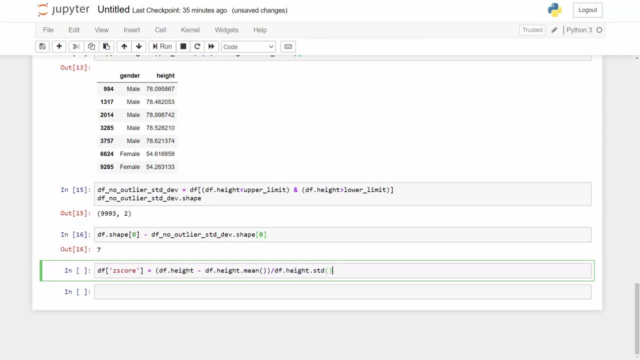 which is a numpy array, and then dot std can give you the second one, but you don't want to use a standard deviation. and once that is done, you can print a couple of samples and you will find that now I have a new column called z-score and I see all these. 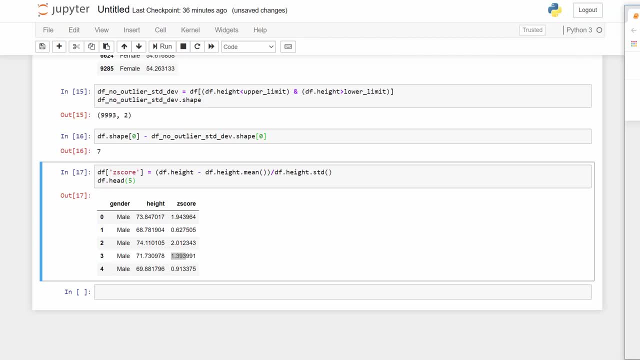 z-scores here. now you can filter out those rows which has a z-score of 3 or above, or minus 3 or below. okay, so the z-score 3 means 3 standard deviation. so you are basically doing exactly same thing that we did here. ok, 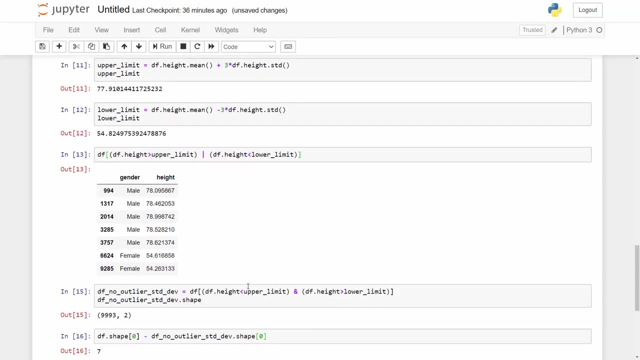 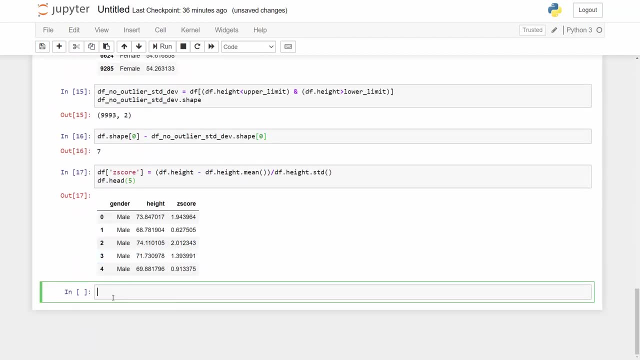 so if you don't want to use z-score and use this technique, fine, you can stop watching this tutorial, but z-score is just an alternate way of doing the same thing here. okay, so here let's say I got z-score 1.94 for this data. 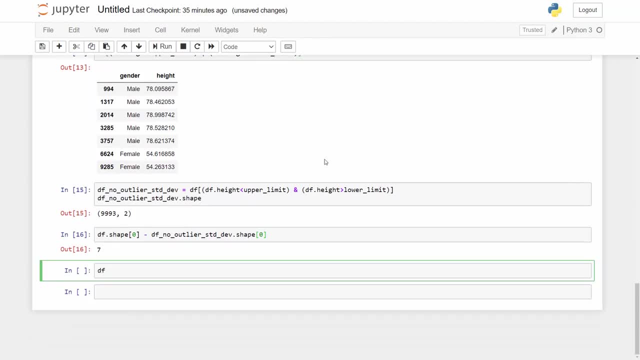 To calculate the z-score. I am going to create a new column in my data frame, call it z-score, and You might know that this is how you can create new columns in the data frame. Okay, and this will be dependent on my height minus height. 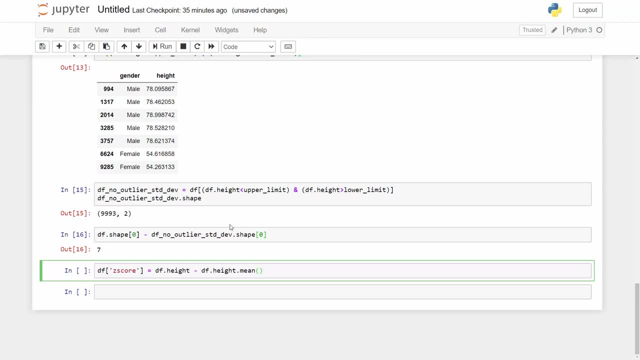 mean. Okay, so it's like X, which is your, this data point minus mean, Divided by the standard deviation. and this is how you can get standard deviation: df, dot height gives you a column in the data frame, which is a numpy array, and then dot std can give you the standard deviation and 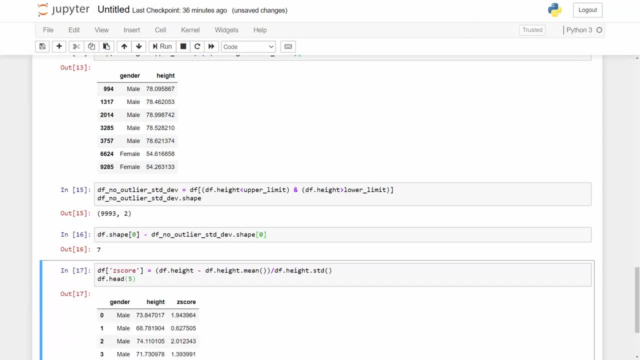 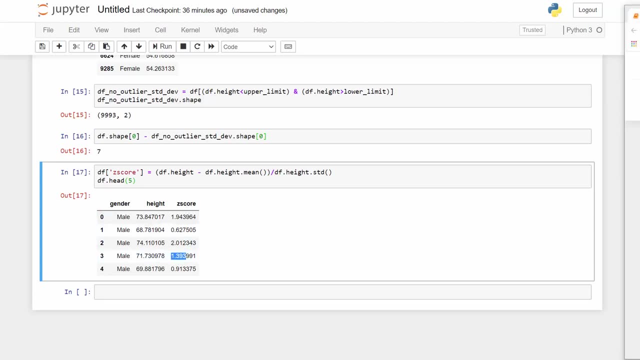 once that is done, you can print a couple of samples and you will find that now I have a new column called z-score and I see all these z-scores here. now you can filter out those rows. which has a z score of 3, 3 or above, or minus 3 or below. okay, so the z-score 3 means 3. 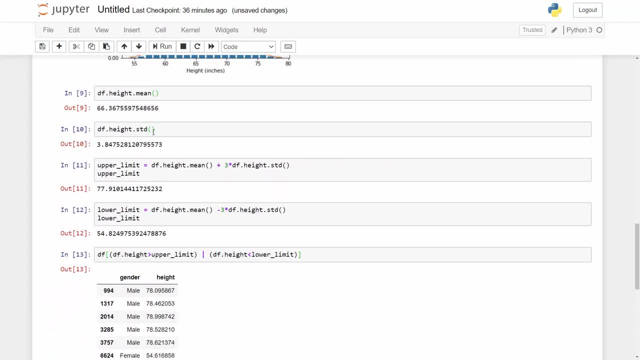 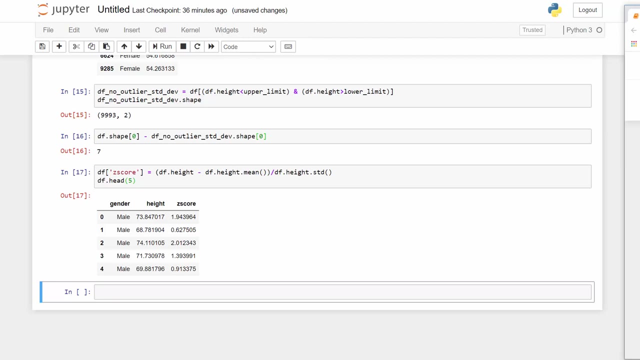 standard deviation. so you are basically doing exactly same thing that we did here, okay so. so if you don't want to use z-score and use this technique, fine, you can stop watching this tutorial, but z-score is just an alternate way of doing the same thing here. okay, so here let's say, I got z-score 1.94 for 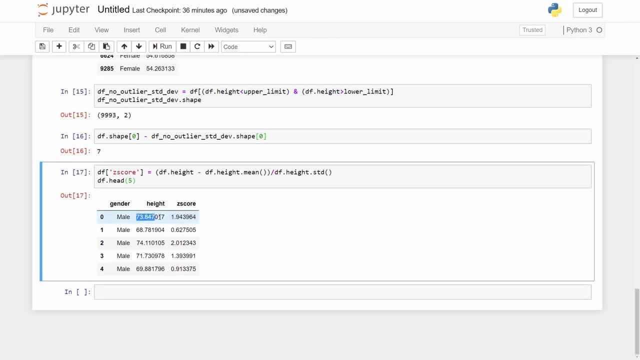 this data point. how did I get it? well, all you do is you take this data point minus the mean. okay, now, what does it mean? is the mean? well, the mean is 66.37. so you did this and you divided that by 3.84, which is your. 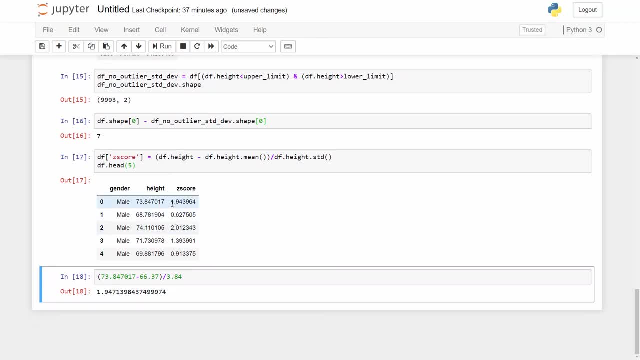 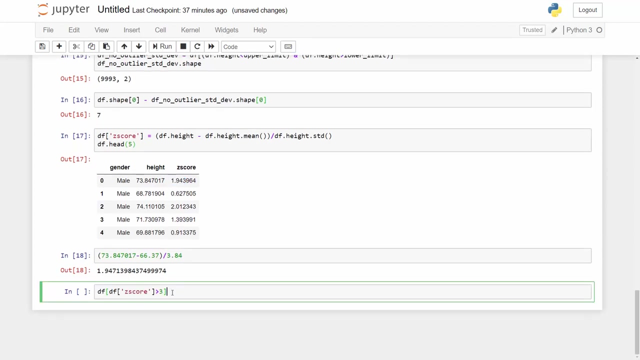 standard deviation, and that's how you got this 194.. pretty simple, okay, nothing to worry about. now i will figure out all the data points which has a z score more than three. okay, this is how you can get all the data points with z score greater than three and you see, you got those. 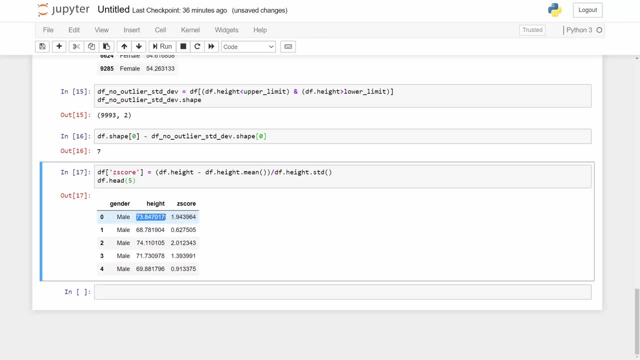 point. how did I get it? well, all you do is you take this data point and you simply apply, or you get this value. you did just click on this point and you can see that animation also pulled up. you can see the tumble minus the mean. okay, now what is the mean? well, the mean is 66.37. so you did this and you divided. 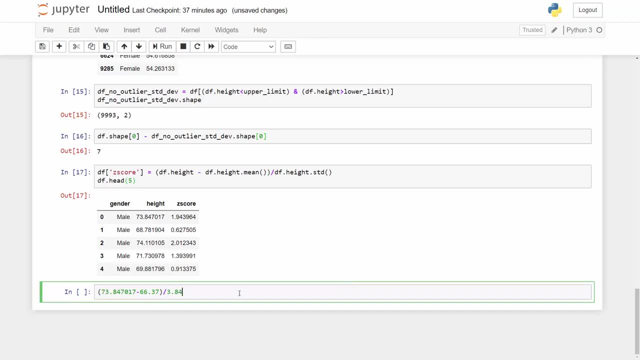 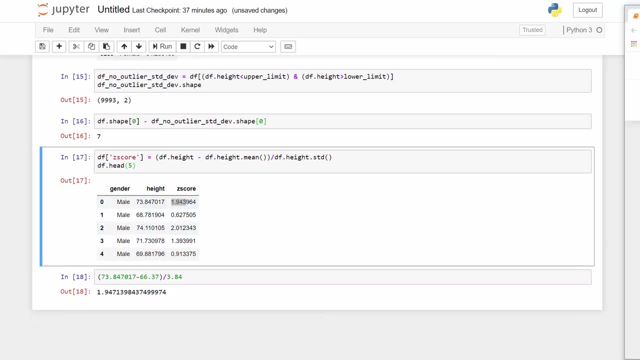 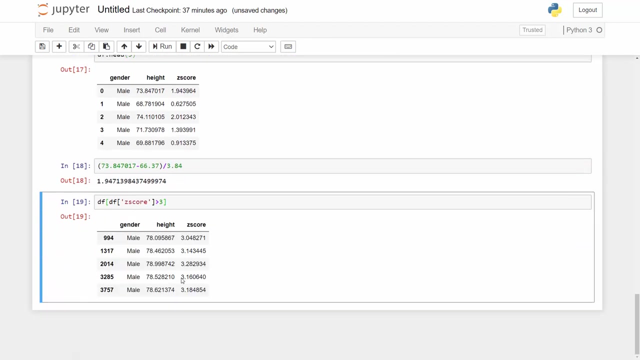 that by 3.84, which is your standard deviation, and that's how you got this 194. pretty simple, okay, nothing to worry about. now i will figure out all the data points which has a z score more than 3. okay, this is how you can get all the data points with z score greater than 3 and you. 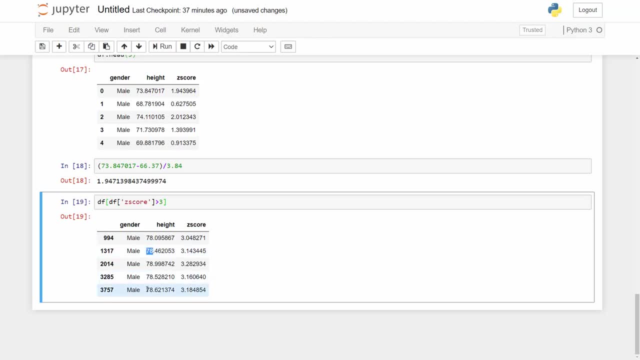 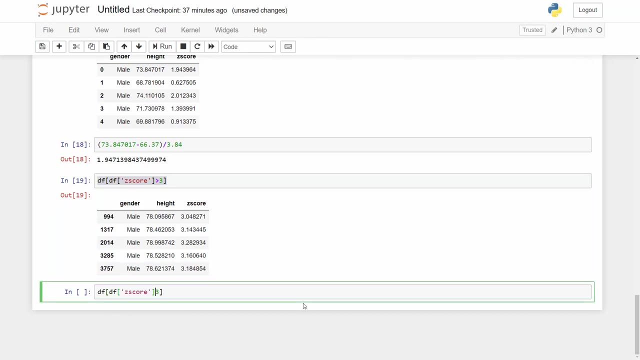 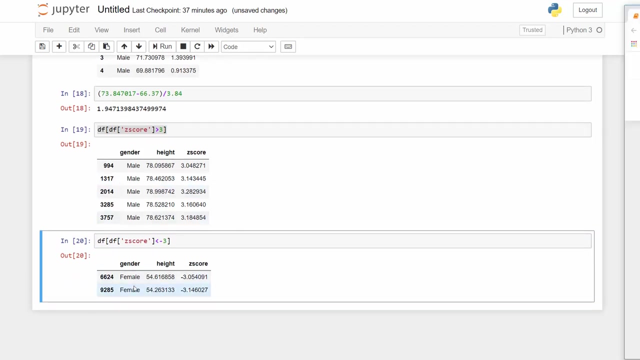 see you got those same 78 inch data points. similarly, if you do z score less than minus 3, you will get these two data points. okay, so 5 and 2, 7. these are the same same outliers that you saw here, so those outliers can be filtered in one shot, or or let's first view all those outliers. 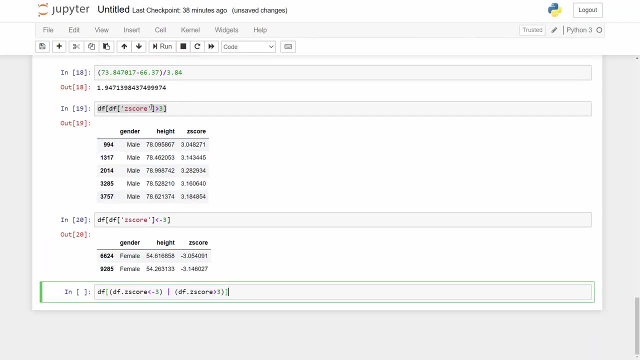 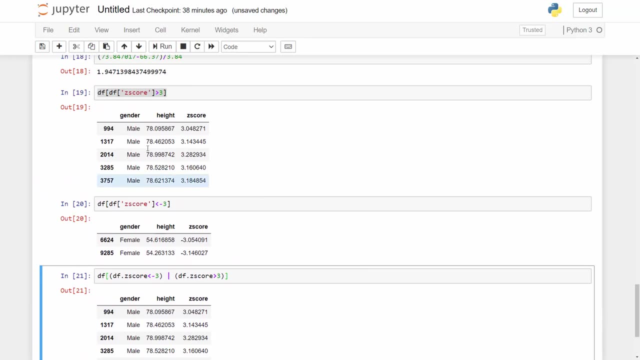 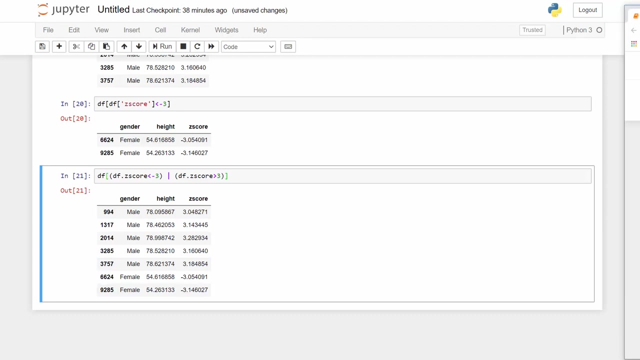 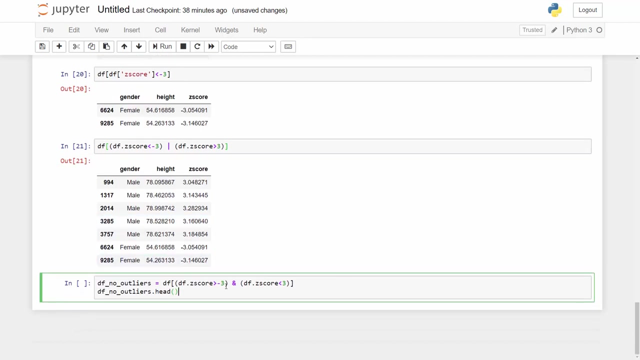 by having this condition. so i'm just doing, or on these two conditions, so that it will show both of them. it's a union of both of these sets and you see these seven outliers. and to filter these outliers again, you can use the same approach that we did previously, which is, uh, you can say: okay, i want to keep those rows. which has 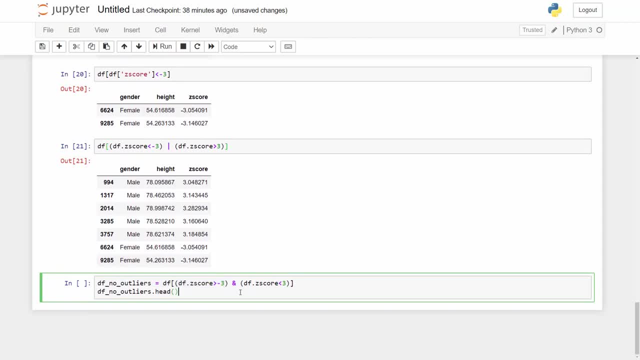 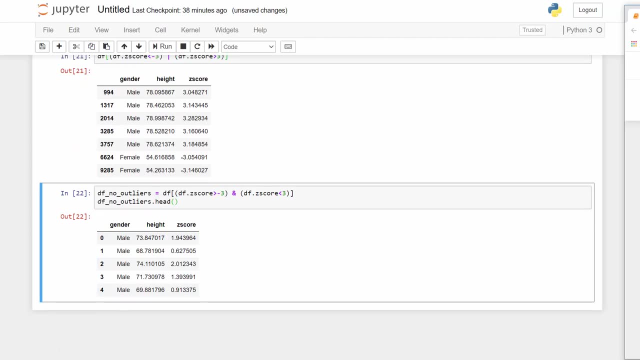 z score greater than minus 3 or less than 3, and you will find this will be your new data frame and in this data frame, when you do something like this, where you are saying df, dot, shape zero, will give you the number of rows in the df and the. this is the new. 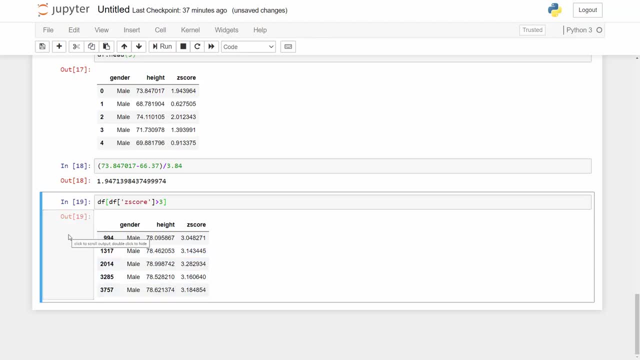 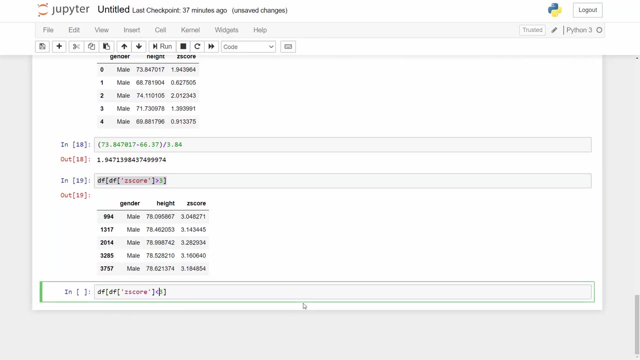 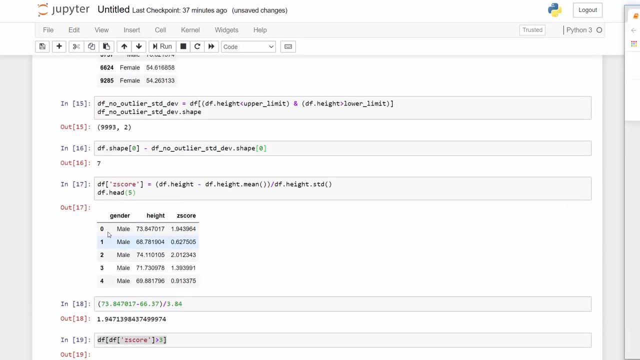 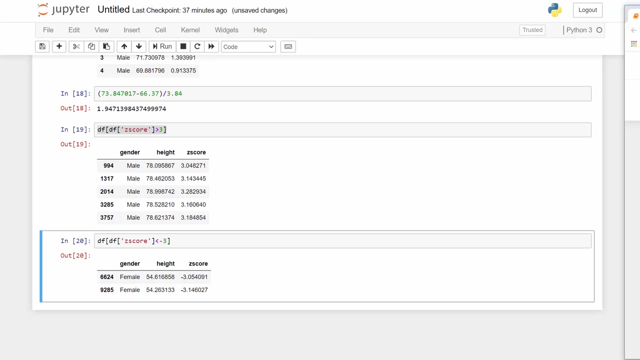 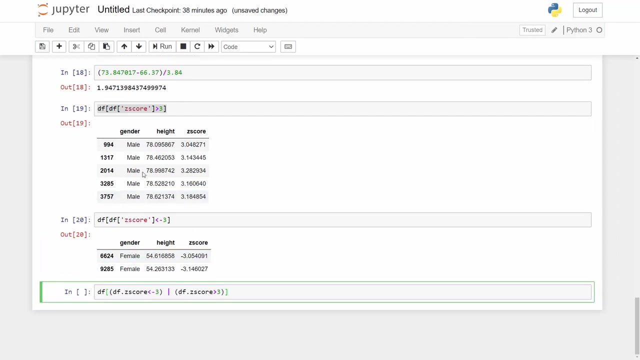 same 78 inch data points. similarly, if you do z score less than minus three, you will get these two data points. okay, so five and two seven. these are the same same outliers that you saw here. so those outliers can be filtered in one shot, or or let's first view all those outliers by having this condition. so i'm just doing r on. 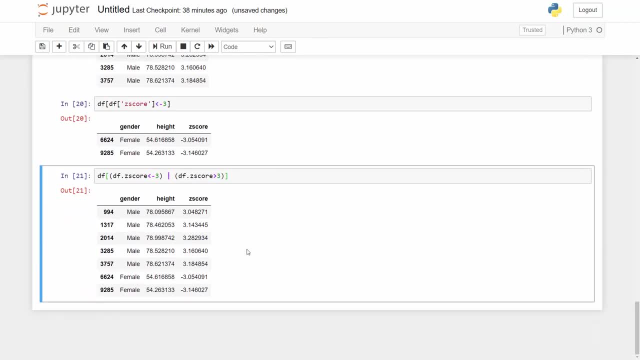 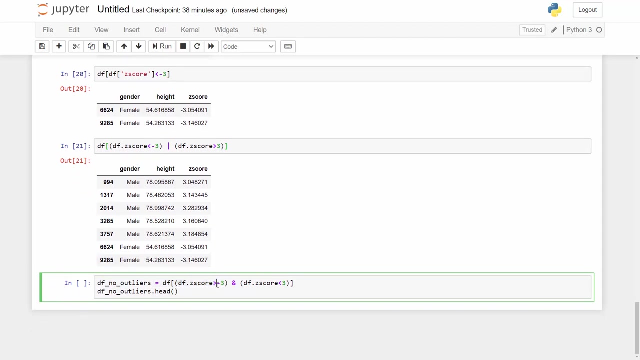 these two conditions so that it will show both of them, it's a union of both of these sets, and you see the seven outliers. and to filter these outliers again, you can use the same approach that we did previously, which is, uh, you can say: okay, i want to keep those rows which has z score greater than minus three or less than three. 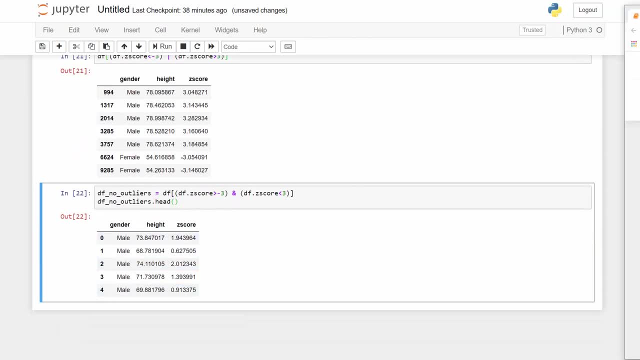 and you will find. this will be your new data frame and in this data frame, when you do something like this, where you are saying df, dot, shape zero, will give you the number of rows in the df and the. this is the new data frame that you have and the rows in that. 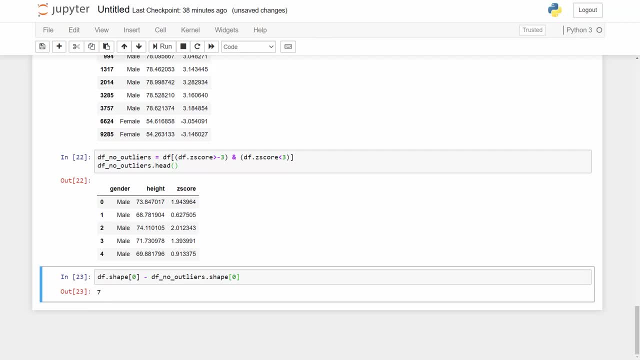 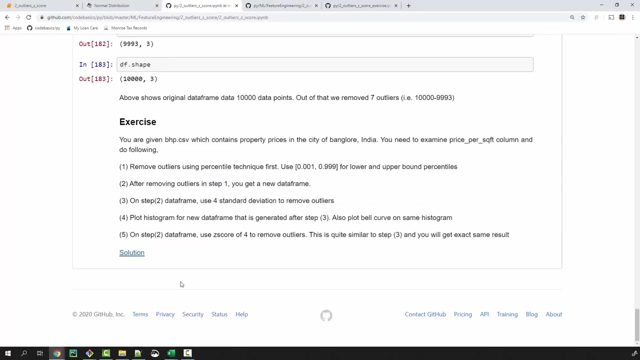 and you find that you removed seven outliers in total. all right, that's all i had. now is the time for exercise, and for the exercise i have this particular uh data set for you: the bangalore property prices. so let me open that. so this is the data set i have for you. 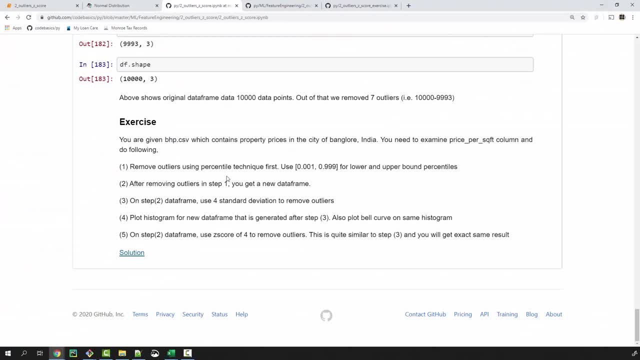 and what you need to do is, uh, first remove the outliers using the percentile technique and then, uh, you get a new data frame. now, on that data frame, you have to use four standard deviation to remove the outliers, then plot histogram, and then you use z score of four. 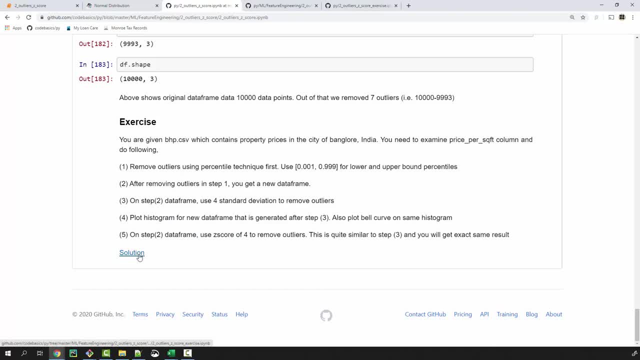 to remove the same outliers. now i have a solution link here, but please try it out on your own first and then only look at the solution. the link of this particular notebook i'm gonna provide in a video description so you can look at the notebook for the solution link and then look at the solution. 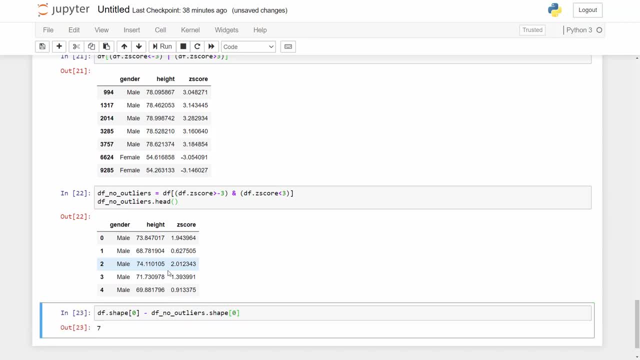 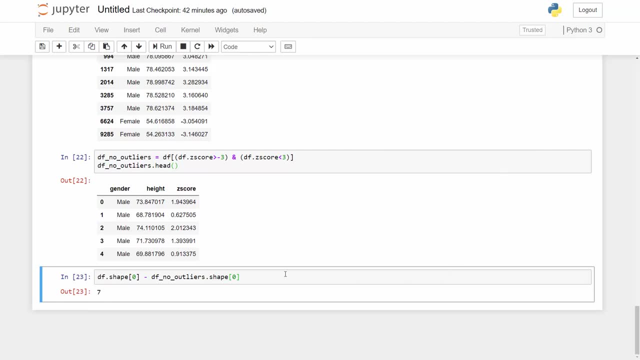 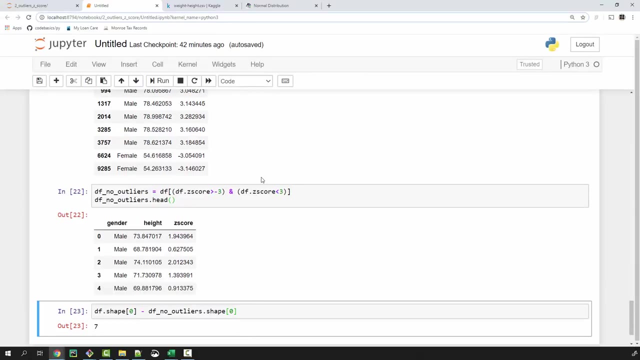 data frame that you have and the rows in that, and you find that you removed seven outliers in total. all right, that's all i had. now is the time for exercise and for the exercise, i have this particular uh data set for you: the bangalore property prices. so let me open that.